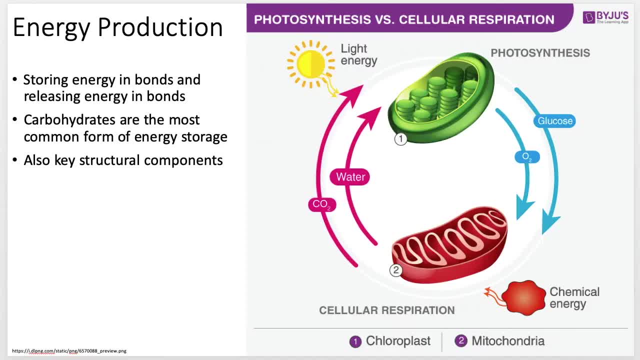 Hey guys. so this week we're talking carbohydrates. Let's get into it. So carbs are our key molecule into energy production. So plants make carbs- ie sugars- and we consume them. to burn those sugars, break those bonds, get the energy out. So that's really. 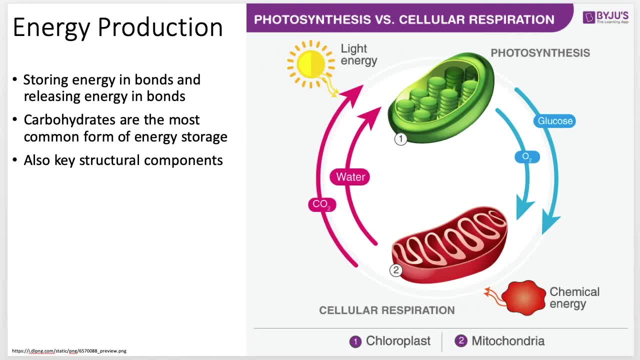 the cycle that's going on. Now, of course, you can substitute in other things. It doesn't have to be glucose, right? It doesn't have to be that. It doesn't have to be. I mean, it does have to be. 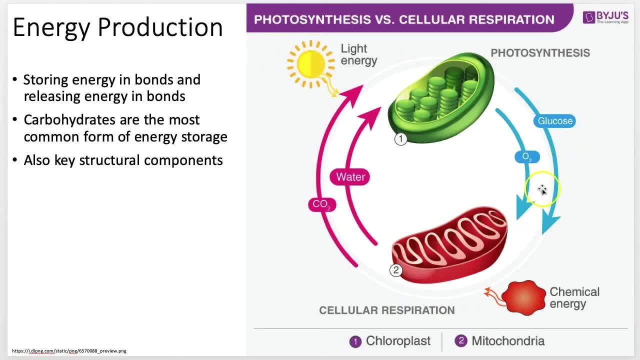 oxygen for the most part if you're going to do cellular respiration- but it doesn't necessarily have to be, It just usually is. If you've taken microbiology, you learn that oxygen is the terminal electron acceptor for many organisms. It's not the only one, but for the most part. 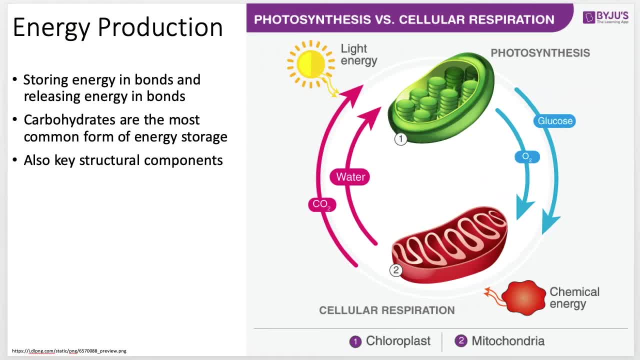 you're going to use oxygen, you're going to burn some glucose, you're going to break some bonds, you're going to get some stuff out, but I have to make those bonds too. So we need to talk about carbs, because they're an awesome, great form of energy storage. Now, that's not their only job. 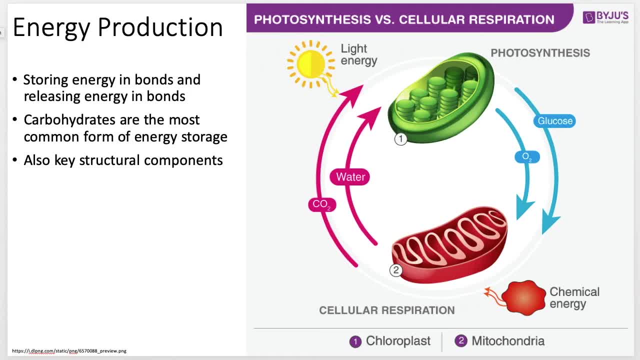 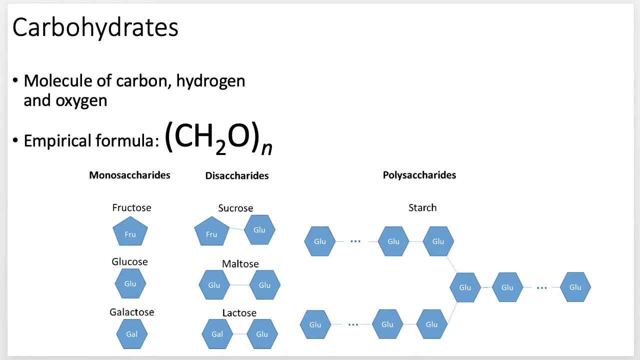 They also serve as an important structural component, And so we're going to talk about that. Okay, Let's talk about the actual name of carbohydrates. So the term carbo obviously means carbon And then hydrates refers to the idea that, if you look at the empirical formula for a carbohydrate, 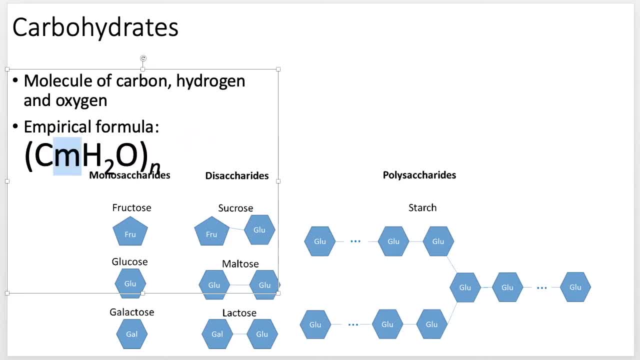 sometimes you'll see a little M here too. I can put it in here, because that's not entirely true- that it's that N, that the number of carbons will match the N. Sometimes you can have extra carbons, but I left it off because hey what? But you have carbon and then hydrogens and octogens. Okay. 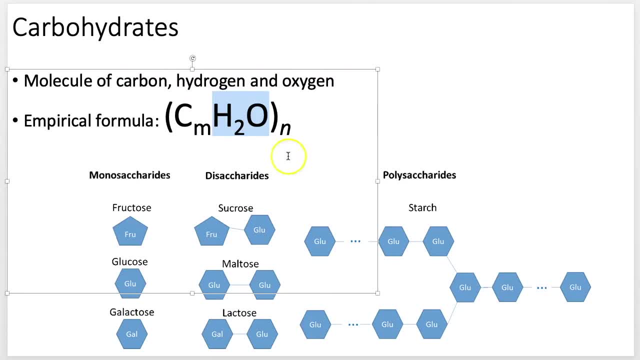 That's your carbohydrates, And so we kind of usually write the structural formula this way, And that lets us it looks like water. So hence hydrate, hydration. Okay, That's why it's called carbohydrates. We're going to talk about all these things. We've got monosaccharides and 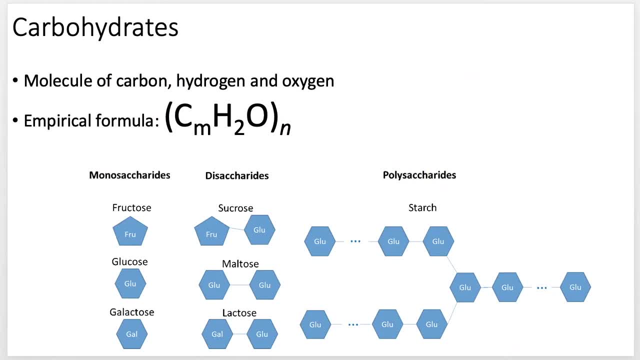 disaccharides and oligosaccharides are not included here- And then polysaccharides. they're going to cover all kinds of cool things. So I'm going to use a piece of a video right now that shows just some of the basics, just going to get our brain. 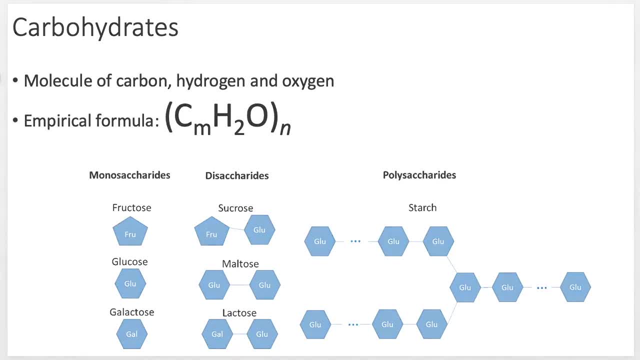 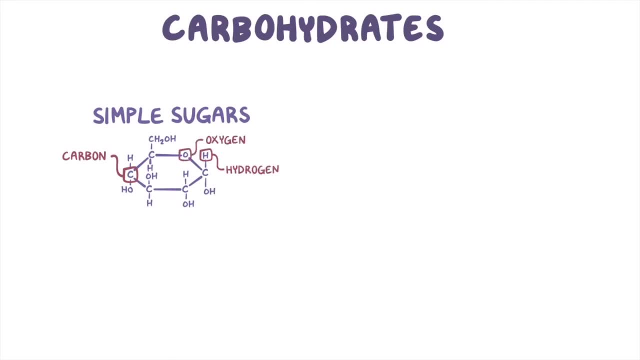 thinking about carbohydrates. It's really really good. Carbohydrates include both simple sugars, which are little ring-shaped molecules made of carbon hydrogen and oxygen, either alone or in pairs, as well as more complex carbohydrates, which are formed when these rings link up together to make long chains. 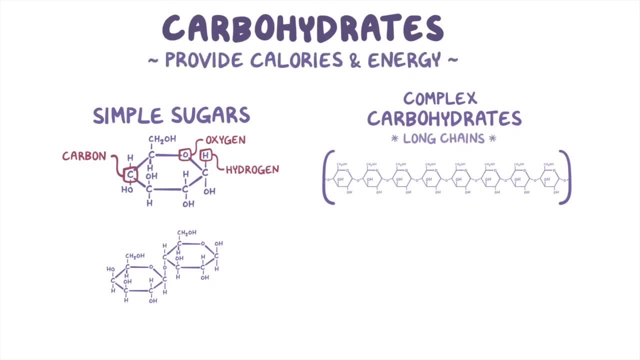 Carbohydrates provide us with calories or energy, and simple sugars in particular play a lot of roles in our diet. They sweeten lemonade, balance out our diet and help us lose weight, So it's really really good. Carbohydrates are also found in acidic miso, soup, fuel, yeast in rising dough and alcohol. 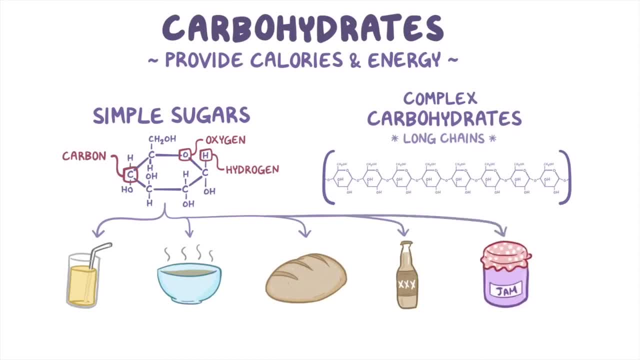 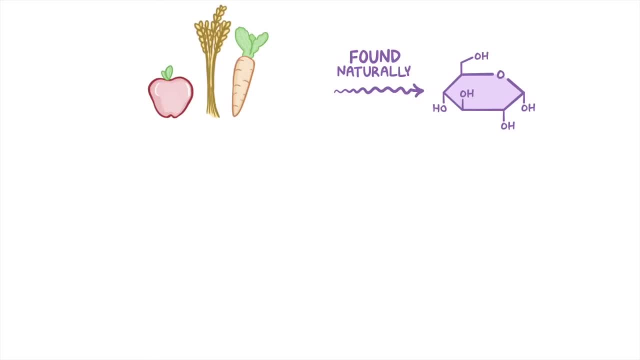 and help preserve jams and jellies. Now, sugars are found naturally in plants like fruits, vegetables and grains, as well as animal products like milk and cheese. Added sugars are the sugars that get added to foods like cereals, ketchup, energy bars and even salad dressings. To be clear, even if the sugar being added comes, 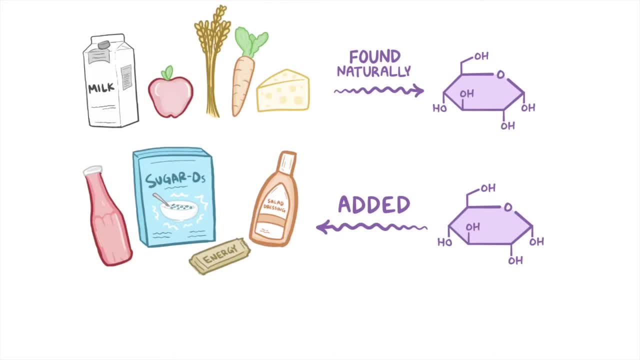 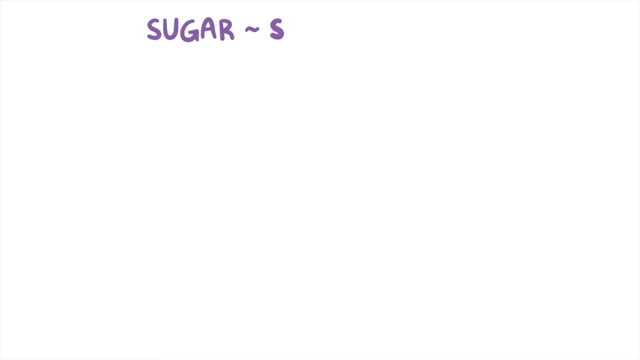 from a natural source, like sugar, cane or honey, it's still considered an added sugar. In fact, a variety of ingredients listed on food labels might be sources of added sugars, some of which you're probably familiar with. Sugar actually refers to a family of molecules called saccharides. 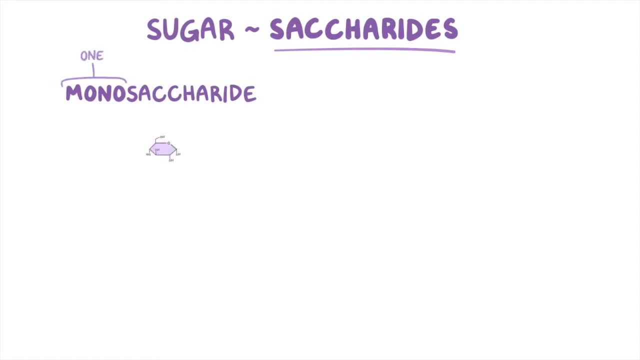 Monosaccharides, where mono means one, so one sugar molecule. Disaccharides, where di means two, so two sugar molecules linked together. Oligosaccharides, where oligo means a few, so it's three to nine sugar molecules linked together. 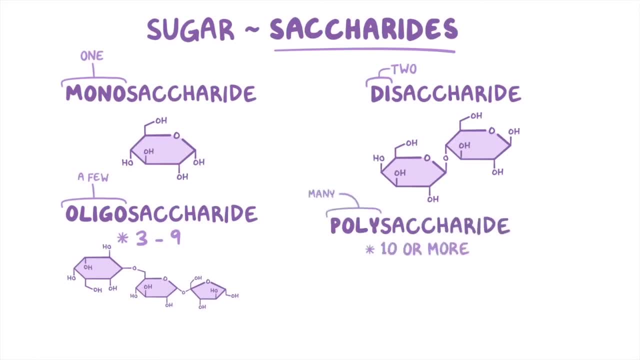 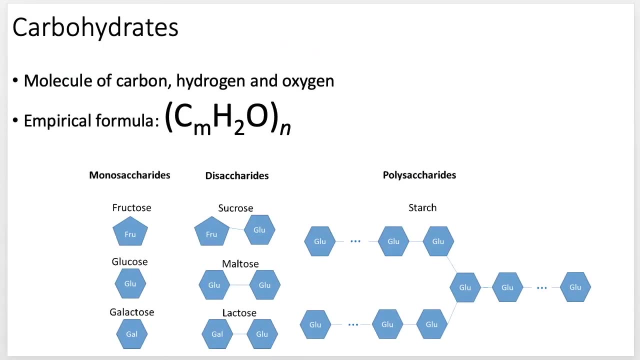 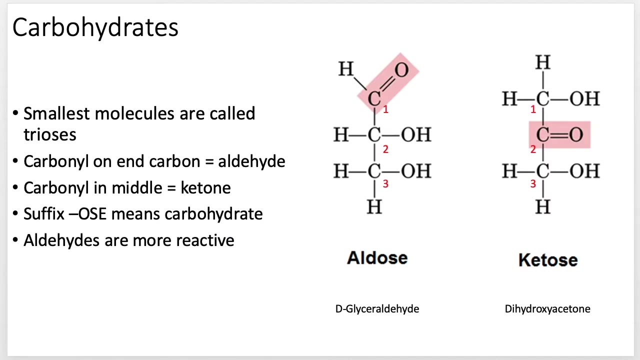 And polysaccharides- where poly means many, so it's ten or more sugar molecules linked together- is from osmosisorg. They make really good videos. We're going to watch a portion of the rest of the video in a minute, So let's start talking a little bit. just some of 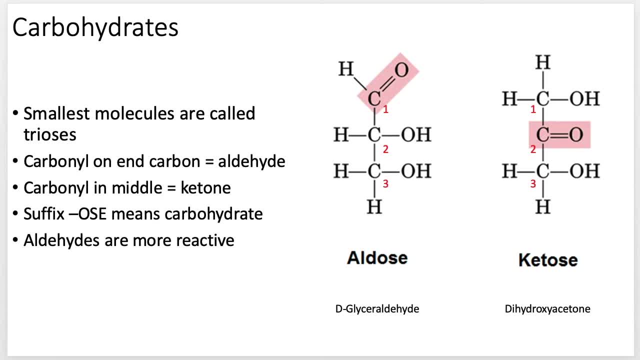 the basics of our simpler carbohydrates. So our monosaccharides are what we're going to start with. So, but first we need to understand just the basic structures and how we're going to talk about carbohydrates. okay, So the smallest molecule that we can actually call a carbohydrate is called a triose. 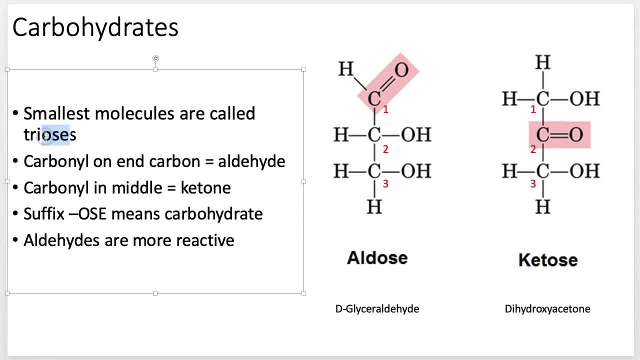 And O-S-E. we're going to encounter a bunch so as a suffix, So O-S-E is a suffix. That's what we call carbohydrates, right? So galactose, fructose, glucose, So if it ends in O-S-E it's a carbohydrate. 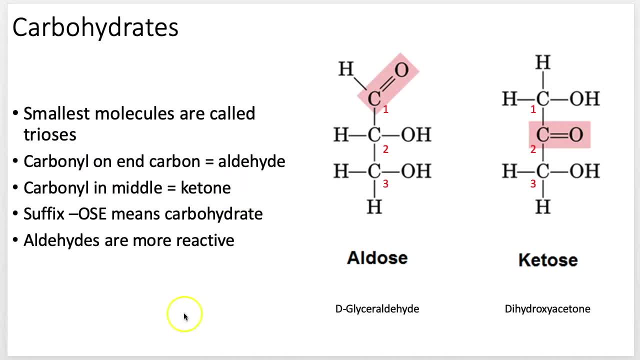 Now, carbohydrates can fall into two different categories. They fall into either aldoses or ketoses, and that has to do with whether or not they have an aldehyde, which is their carbonyl on the end, or whether they are ketones, where 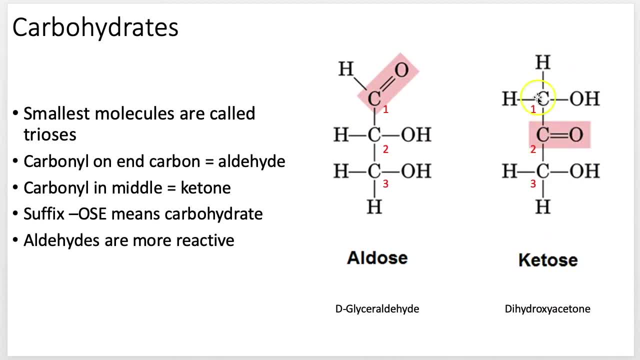 they have their carbonyl group stuck somewhere in the middle, not on one of the terminal carbons. okay, And so that's how we organize these. Now, most of the carbohydrates that we're going to encounter are actually aldoses. Why is that? 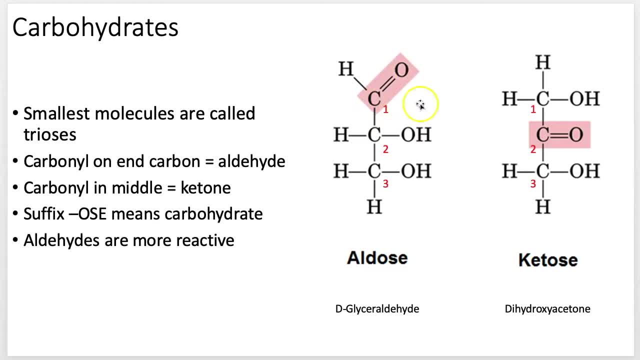 Well, it turns out when you have an aldehyde. so when you take that carbonyl and put it on the end here, it's easier to, It's easier to react with than if you have all these other things kind of blocking this. 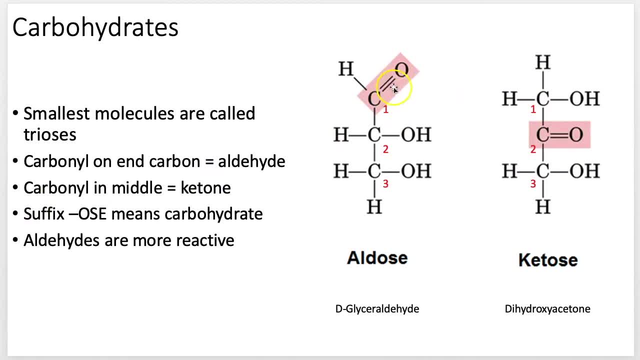 double bond, And so you can just kind of physically imagine it's easier to get something into this space here to react with this bond to form something else. So like I could roll this guy, attach it to the other end of this molecule which I'm 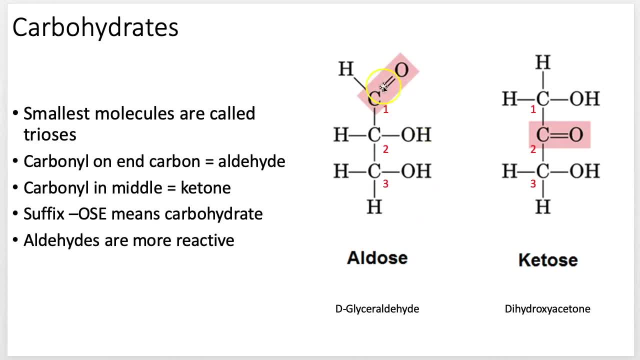 going to show you in a little while. I could attach it to something else and just modify it, or I could come over here and cleave that bond and it would be easier. So aldehydes in general are more reactive. They're more reactive than ketones because they have these extra carbons on the side. 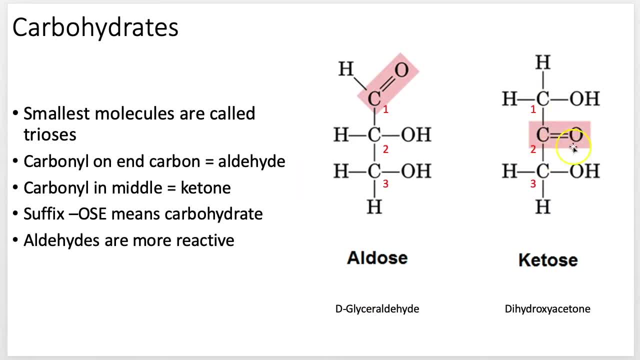 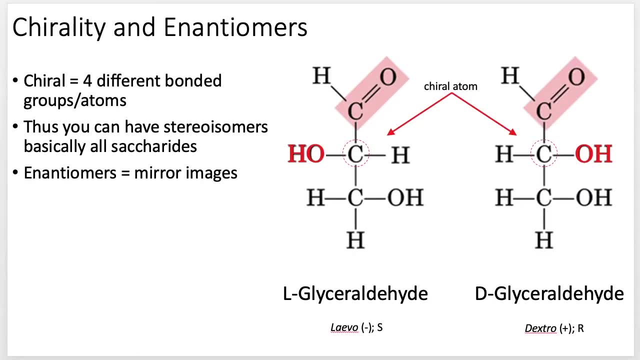 are sort of protecting. the reactivity of this carbonyl group here Leads into the idea that comes up a lot with sugars and carbs and stuff is the ideas of chirality and enantiomerity or enantiomers. So a little organic chemistry in here, but it's not that bad. 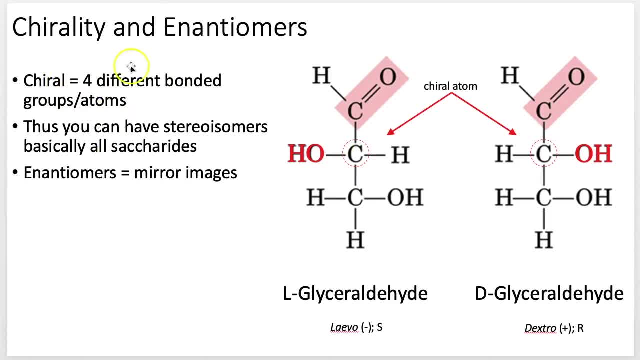 So what does it mean to be chiral? Well, that means Practically, it means that you have a carbon with four different types of groups attached to it, And so here we have our aldehydes, So it's one of these. 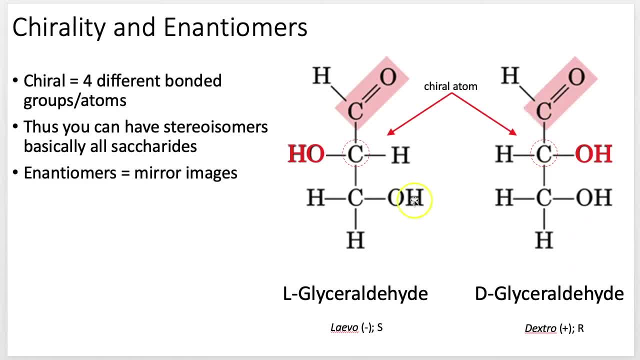 These are D-glyceraldehyde, And here's the difference between D-glyceraldehyde and L-glyceraldehyde. I'm going to talk about that in a second. And so with D, we have the hydroxyl group on this side. 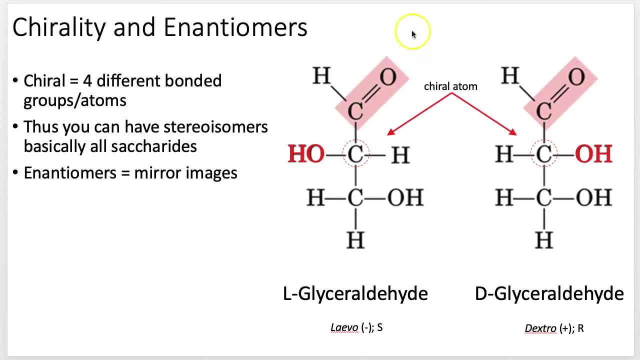 With the L, we have the hydroxyl group on this side And because you have four different things, you have this crazy looking thing here. you have a hydrogen, you have this group and a hydroxide. So because there are four different things, that means that you have a carbon. 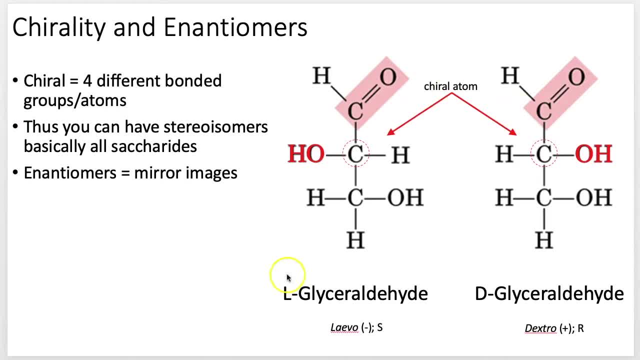 So that means I can sort of have a mirror image. So that's where our chirality, Well at least the chirality of our atom, is concerned, And enantiomers is what we actually call the mirror images. So we can flip these things over. 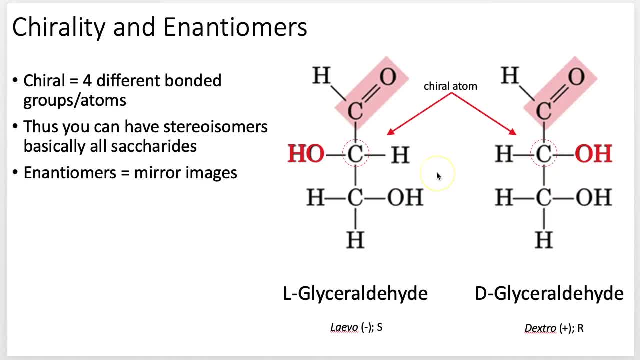 If I put a line down the middle, you can flip these onto each other, So it's like your left hand and your right hand. They have all the same structures, but they're just in different locations, And so that's enantiomers. 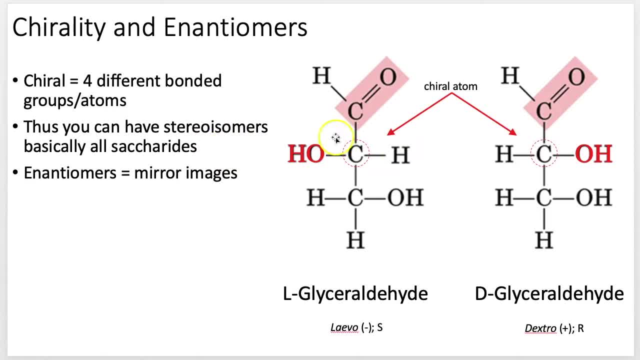 Now stereoisomers, ie if you have chirality, basically all your saccharides, as long as they're aldoses, can engage in stereoisomeric forms. They can have chirality, And we're going to see some examples in just a second. 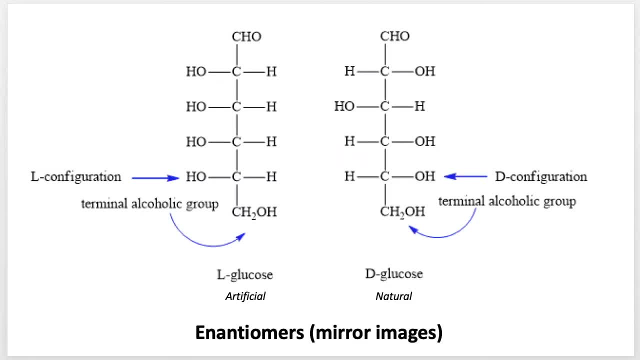 And that can actually have a big effect on what they're used for. Glucose is probably the simplest one to actually look at. So here's glucose. here It's got six carbons, C6H12O6.. Awesome. But how we configure it? because we have chiral atoms. 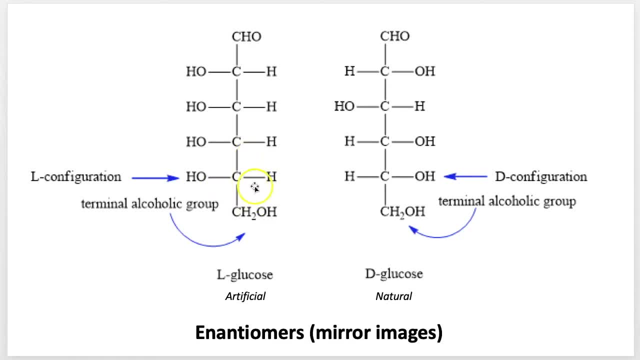 we have chiral carbons, we have multiple chiral carbons. we are able to maintain the location of the R groups or whatever is attached to those carbons, And so you can maintain those And then, as they're folded over or reactions happen, 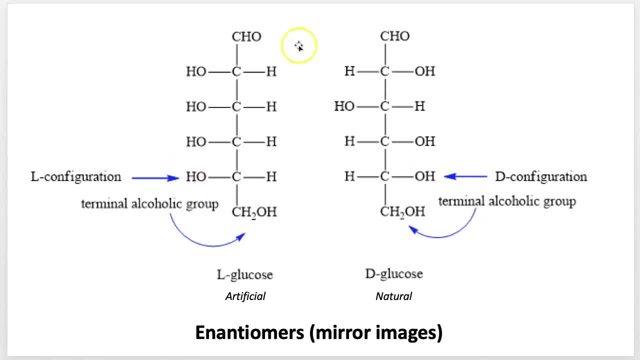 then they're going to maintain their location, even though the content is the same, And so natural glucose looks like this. This is the deconformation, So you have three on the right and one on the left. That's kind of how I. 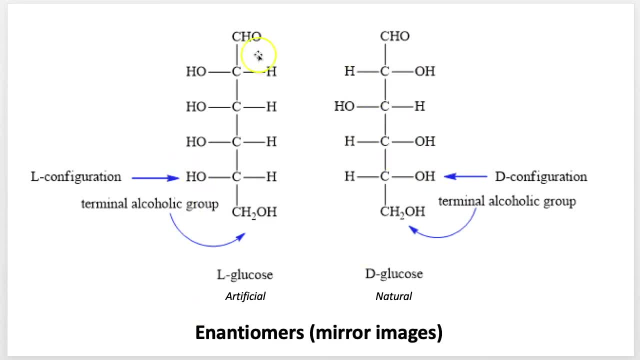 Now, when you artificially generate glucose, it's L-glucose, and all of them are on the left. See that. But we don't really care what the key one here is. We're looking at this chiral carbon here because you can flip them. 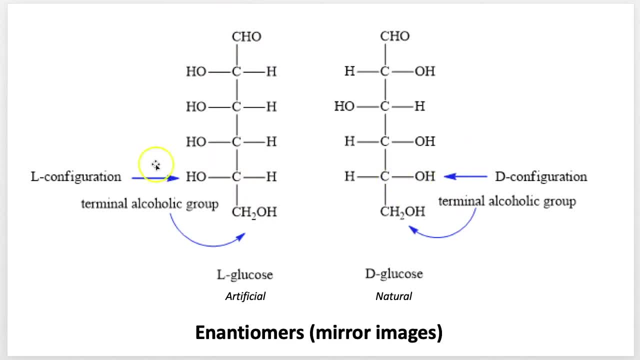 It doesn't really matter. This one is the chiral carbon that decides whether it's L or D, because that's what determines if it's glucose or not. I'm going to show you some later on, If I start flipping some of these hydroxyls. 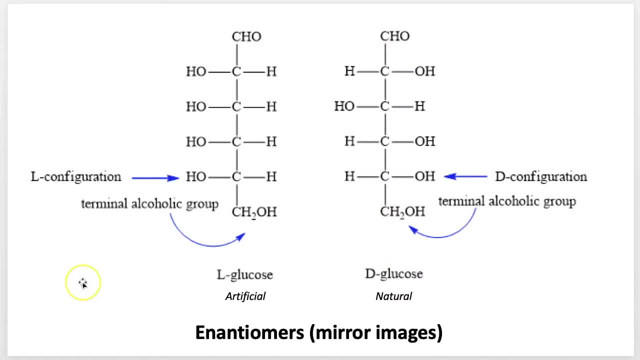 we actually change the name. But you can see, this isn't my favorite thing because it gets really complicated and some of the terms get really complicated, And so I apologize, But honestly it's not too crazy, It's just wherever you put that hydroxyl group. 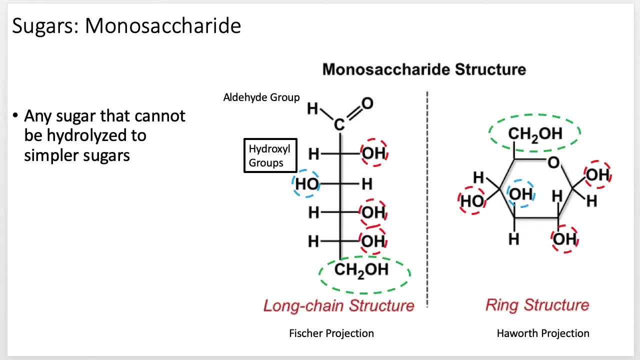 it lets you change the name. It's not that complicated, So let's keep going. Let me just talk a little bit. I've been showing you Fischer projections. So that's when you linearize the carbons, that sort of carbon backbone that the sugars are going to be made of. 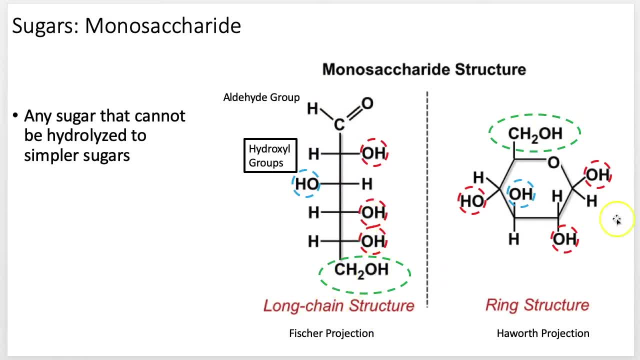 Okay, And if you fold those carbons over on the left, they're going to bond on themselves, Okay. So if we actually form the bond here between, basically, this oxygen is going to go attached to this carbon here, Okay, And so if you imagine that you're sort of like on a plane here, so a PLANE. 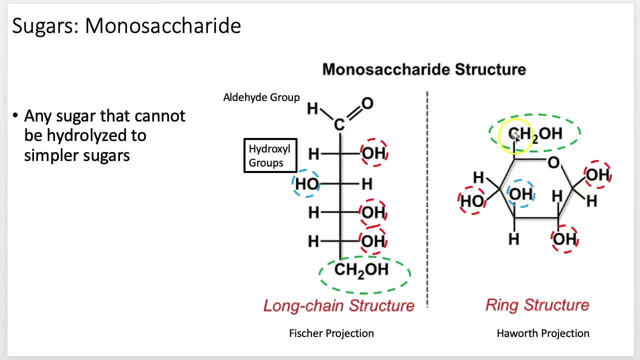 So all the carbons here? so there's one, two, three, four, five, six carbons. These five carbons here are sitting, existing on a plane. Okay, And then, off of that plane, your hydroxyl groups are either going to stick up or they're going to stick up. 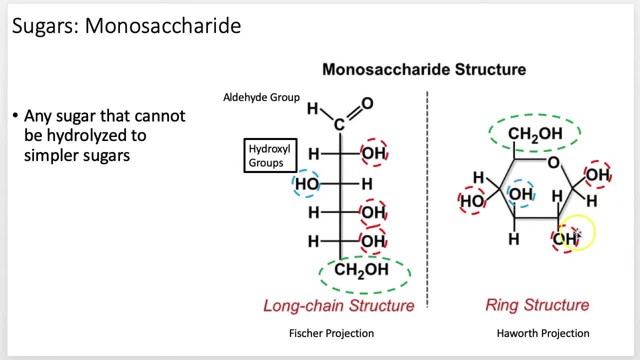 This is actually supposed to be sticking up, So they'll stick up. The blue one's sticking up, and then these red ones are sticking down, So let me show you a better picture here. So we've got our carbons here. So there's our Fischer projection. 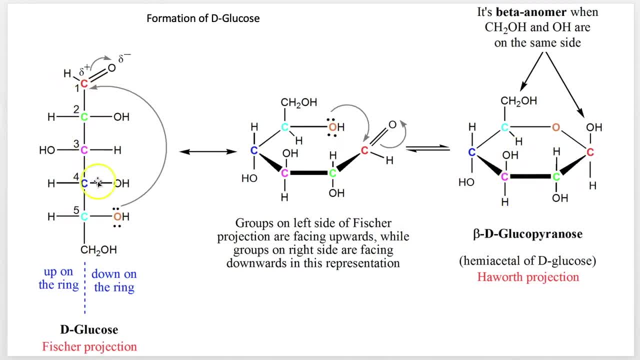 Okay, And they're colored Okay. So there's the red one, the green one, the pink one, the blue one, other blue one, And there's the oxygen. Okay, They were actually formed to this carbon here, Okay, And off of that we can see where. so there's my plane of existence. 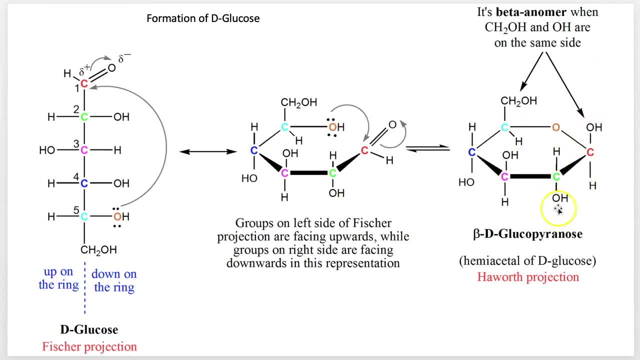 Right, So this is in three dimensions, And so one of the hydroxyls is sticking up, This one's sticking down, This one's sticking up, This one's sticking down. Okay, Up down, up down, And if I change how those are arranged, it can actually change the functionality. 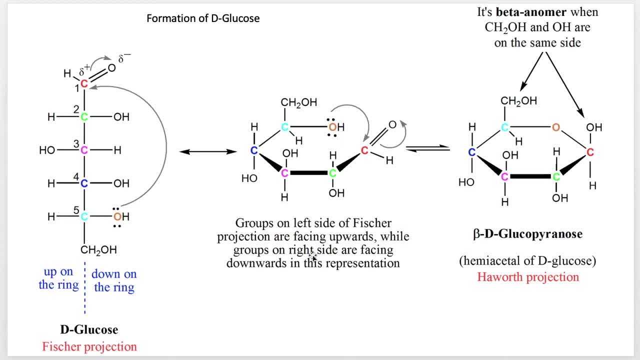 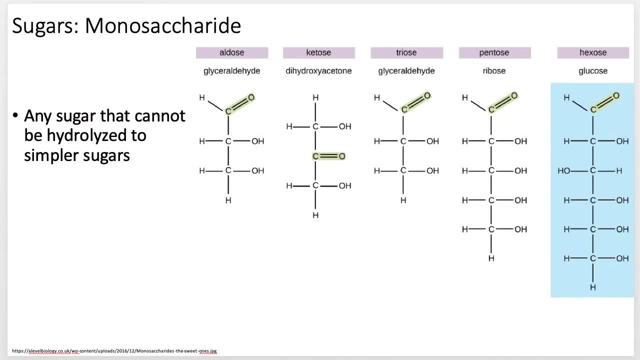 It can change how reactive it is. It can change the actual name that we give them, which is kind of fun, Okay, So let's keep going. There's lots of different monosaccharides. It just kind of depends on how many carbons you're going to include. 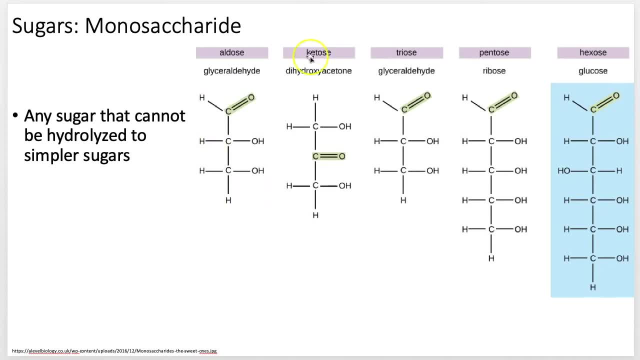 So you have your aldosis and ketosis. So that's your three carboners. Carboners, I just made that up. That's your three carbon molecules, And then, as you add, carbons, so glyceraldehyde is an aldose. 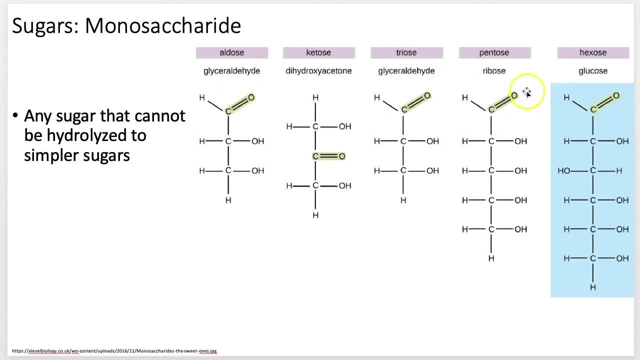 Okay, It's got an aldehyde on the end. Notice, all of these are aldoses. Okay, And then you can also have a ketose which is dihydroxyacetone is a ketone. Now, all the rest of these are aldoses. 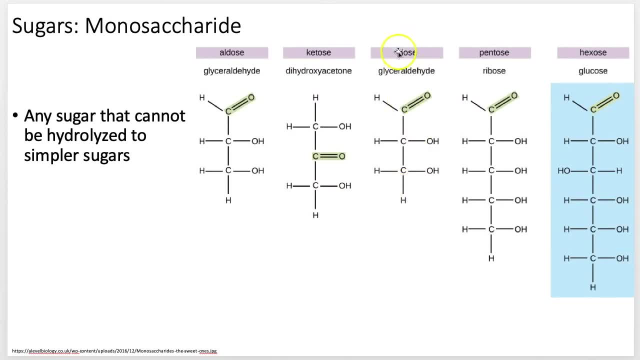 And so the number of carbons decides what number gets up front. So if I have three carbons, it's triose, If I have five carbons, it's pentose, If you have six carbons, it's hexose. 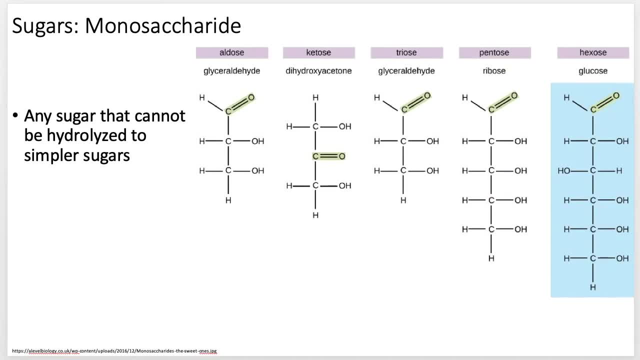 Now, most of the. if you're not doing anything weird, then most of the carbons are dihydroxyacetone And most of the time you're going to be encountering pentoses and mostly hexoses. But hey, sometimes if you're doing weird stuff maybe you'll have a quadros or whatever tetros. 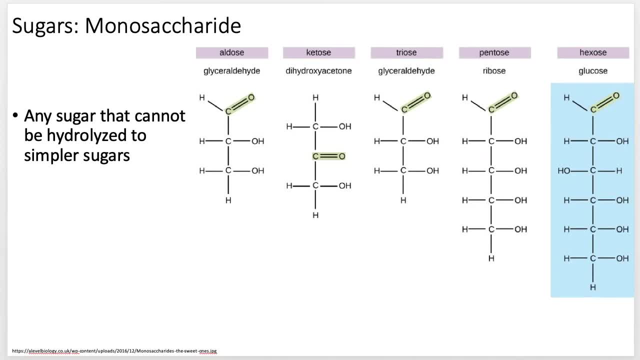 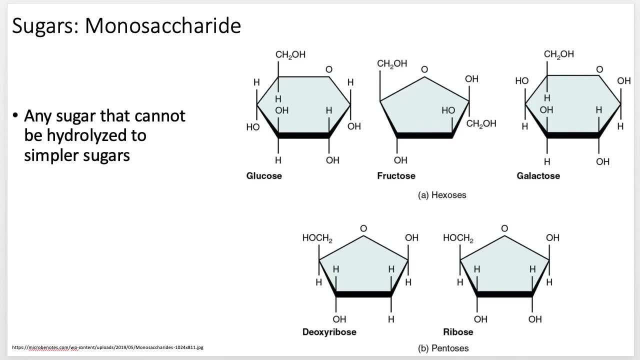 It doesn't even list them because that's like super rare, unless you're doing weird chemistries. But we're going to assume that you're not doing weird chemistries. Now, of course, these are Fischer projections, So we can look at. what do you call these? 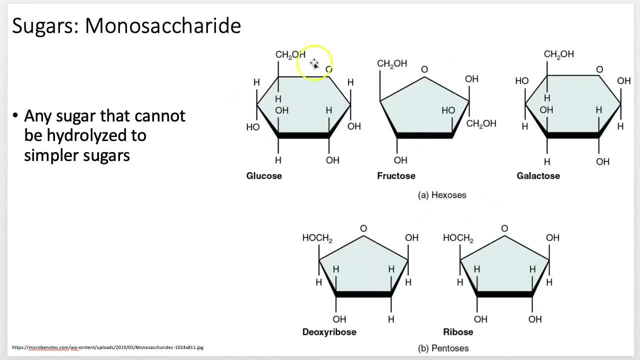 Hayworth projections. Sorry, I forgot. So you can look at the Hayworth projections And so you can just see structurally what's going on, And I have a couple of them. I always center myself on the oxygen, So here's my typical glucose molecule looking right there. okay, 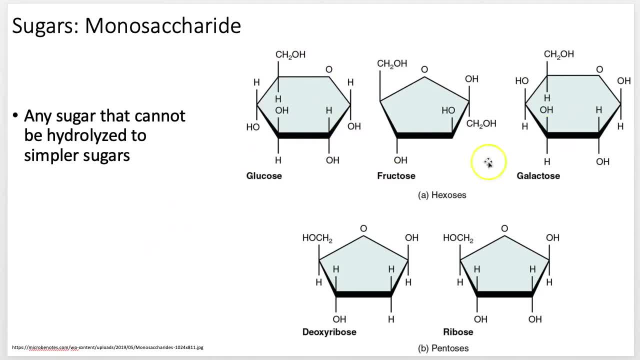 Now, monosaccharides basically are. these three are the monosaccharides that we're going to be dealing with most of the time. Okay, You can have other monosaccharides, okay? So, like riboses and deoxyriboses. 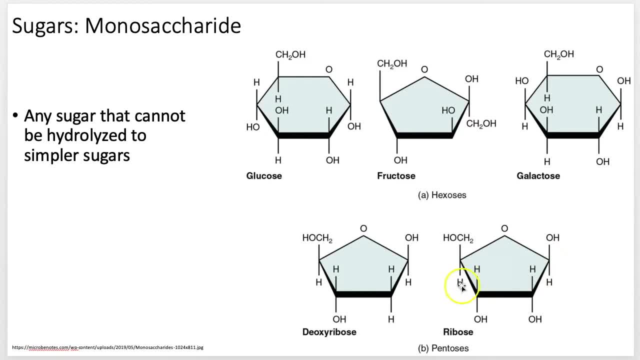 Those are pentoses, right? They only have five carbons, So we got one, two, three, four, five carbons. One, two, three, four, five carbons, right? That's what we use to make our nucleotides. 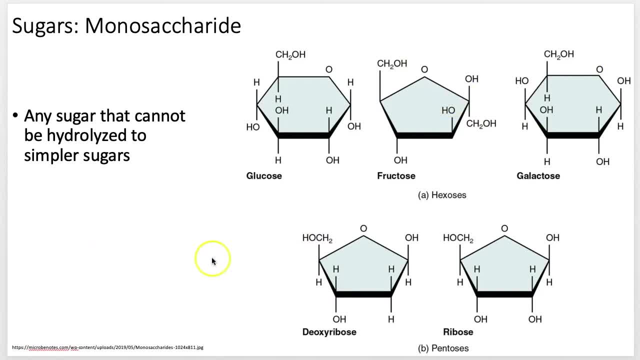 When we're actually making our nucleotides, we're actually making our monosaccharides right. So that's what we're going to be dealing with most of the time. So we're going to be dealing with our carbohydrates Like for energy. then we rely on more, on our hexoses, which have six carbons. 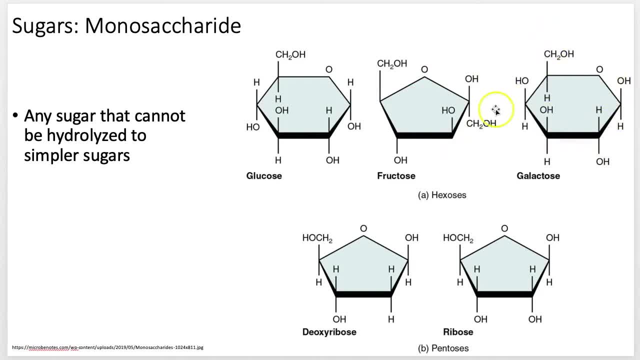 So one, two, three, four, five, and then you get that six one sticking off there. Now for fructose, which is one of the monosaccharides, one of the three. it's a little different. it kind of looks like the pentoses. 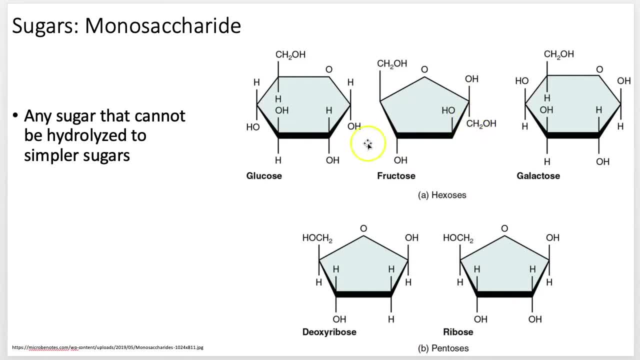 but notice, you got this extra carbon hanging off the bottom here. So sometimes people are like, well, those look the same. Well, they're not actually the same. It's just the carbons Mentioned just a minute ago, that where we put those hydroxyls. 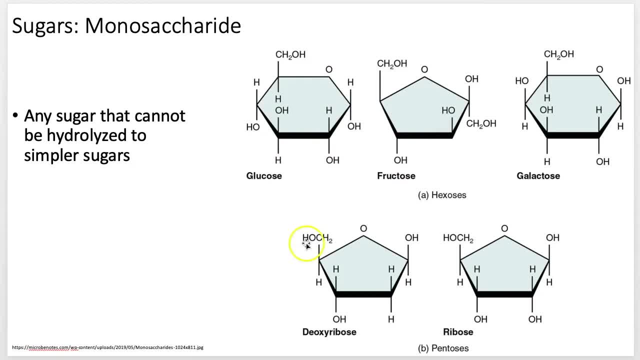 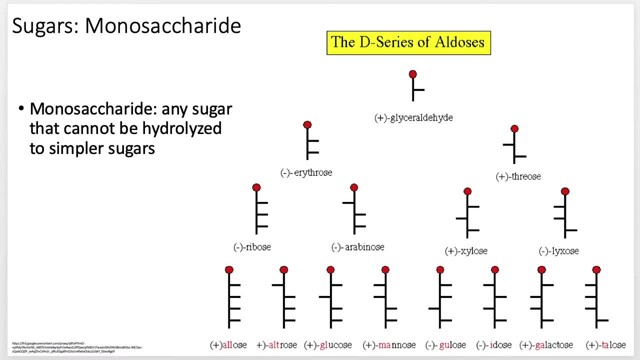 whether they're on the top or the bottom, and I can change where these are on the actual molecule this refers to. we can use those to keep track of the actual types of aldoses that we have. okay, And so you can see the D series. so these are naturally formed aldoses. 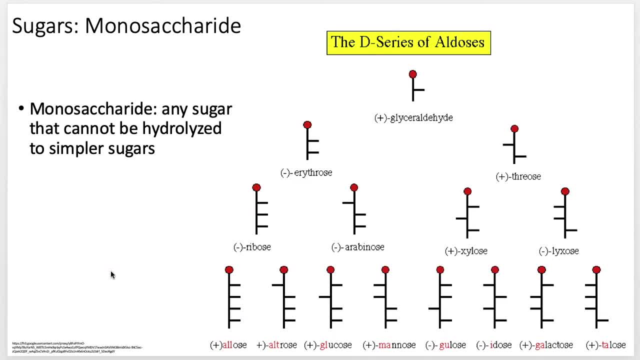 So aldoses, they're aldehydes. This is most of the sugars that we're going to encounter. So you can see down here on the bottom, we've got our lactose glucose and we've got our mannose and we've got our galactose. okay, those are. 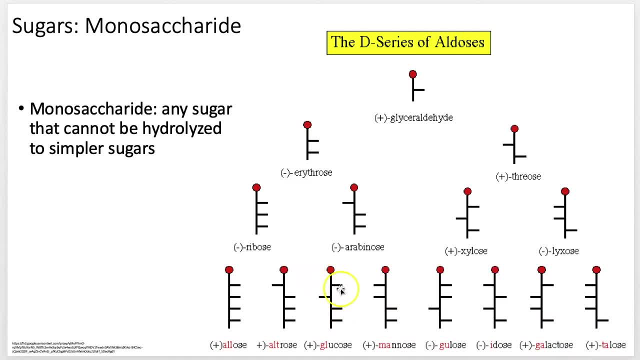 three biggies, okay, and so we've got our. we have three on the right, one on the left, two on the left, two on the right, galactose, two on the left, two on the right, and so you can just kind of see, basically we just change the names based. 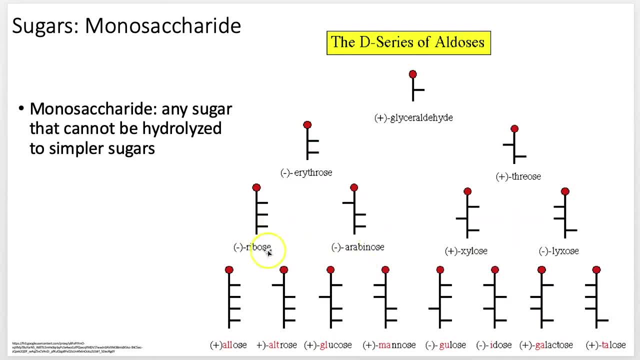 on where these things go. arabinoses show up riboses- there's your ribose, xylose, you'll see sometimes, but there's a bunch of these that just never show up, like goulos, I don't know, it's just really weird. eidos: they're just generally don't get made. you can synthesize them, but for the 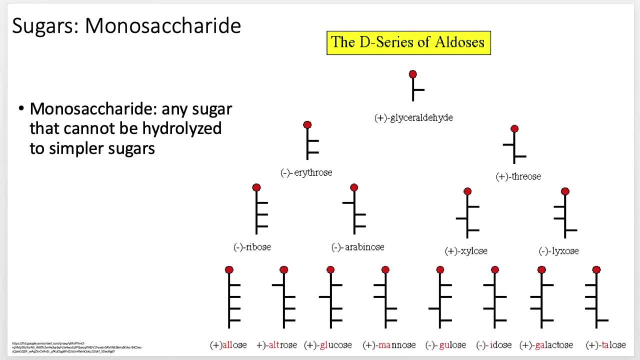 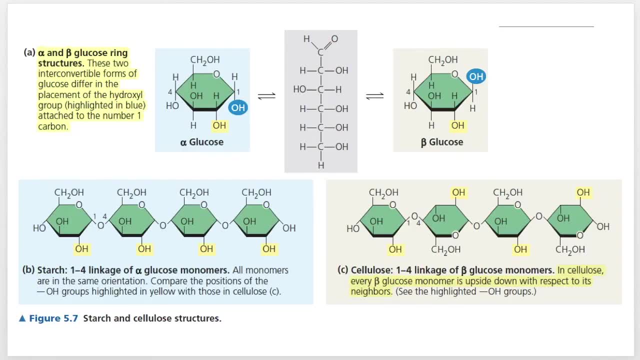 most part, but hypothetically they can exist. and so, yeah, that's what that is. one question gets up all the time: who cares? okay, well, it actually matters because, for example, if I'm going to build like a polymer of sugars, okay, so now we're not talking about polymers yet, but I just want to bring it up because 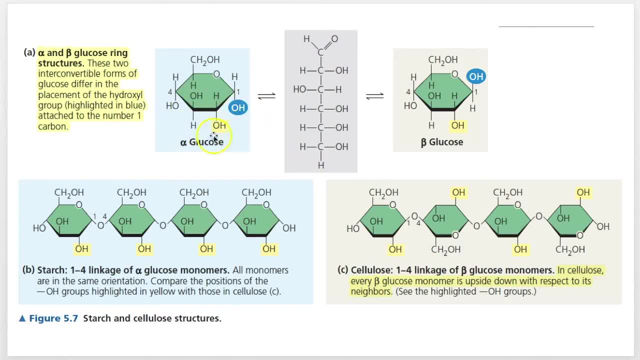 it's a good question. it has to do with where your hydroxyls are, so in alpha glucose. so just to orient yourself, there's the oxygen right. so we're looking at this first carbon here. this first carbon is going to decide our that it's a glucose. oh, sorry that the 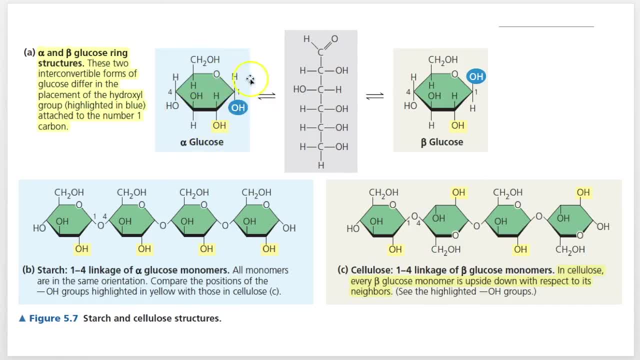 this hydroxyl is down, so it's a glucose, and then we get to flip this one, sorry. so the number two carbon decides if it's a glucose. the number one carbon gets to decide if it's alpha or beta. okay, and so we're gonna look here and we're gonna 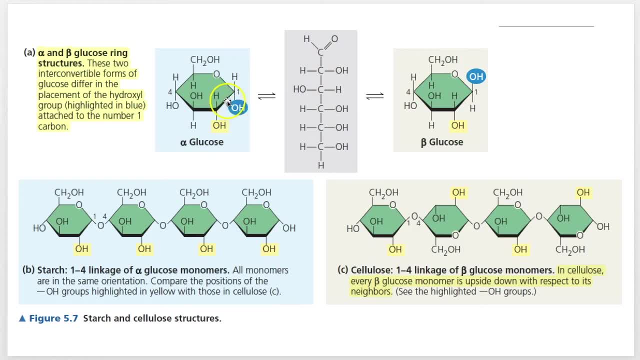 flip our hydroxyl down, that's an alpha, okay. and if I link a bunch of these, a bunch of those, together with glycosidic linkages, which we're about to talk about, then i get this kind of formation of all these alphas. this is a typical formation for starch. 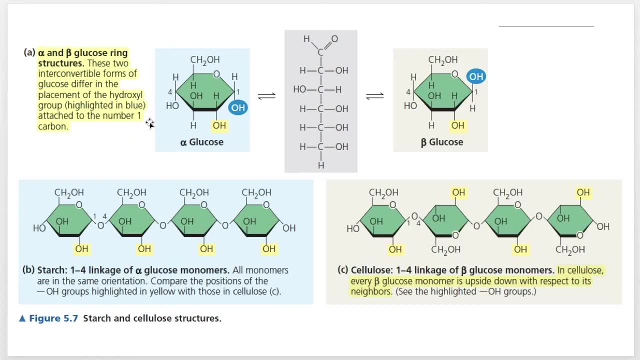 which is a very digestible yet long-term storage molecule. okay, so this would be your starches, so like things that you can eat, like um, uh, i don't know- like, uh, complex carbohydrates. so when you hear complex carbohydrates, this is what they're referring to. there's these long chains of sugars. 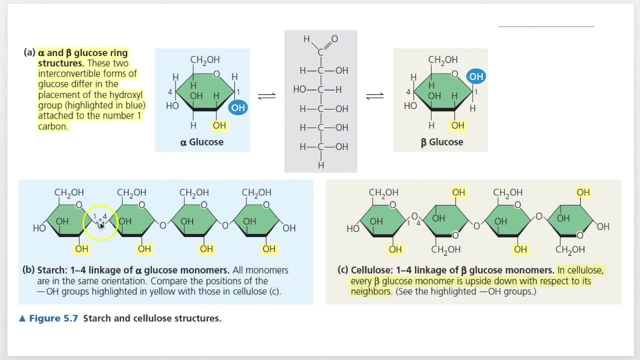 they're not monomers, they're polymers, and so that's what they form, but it's digestible. now the key there is: if i jump over here, okay, i've got all these uh, beta glucoses, so that's where the hydroxyl group is pointing up here, okay, and i'm gonna kind of keep flipping them. so if i keep, 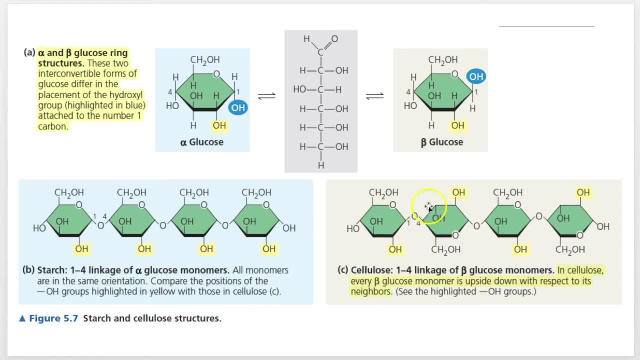 attaching all these betas to each other. uh, you can see they start getting like kind of this weird shape. so in order to get them to actually bond together properly, i have to flip them. so half of them are flipped, and so you see the little blue, the little yellow blue man. 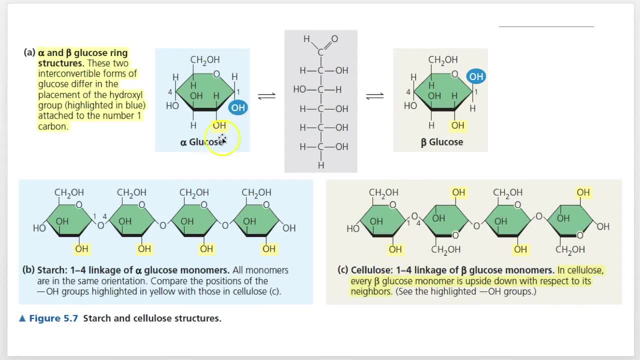 uh, the little yellow hydroxyl groups that determine whether this is like glucose or not, pointing down, up, up, down, up, down, up, uh, in comparison to each other, as these are all down derp, i'm just saying what's really obvious. um, if they're like that, that is. 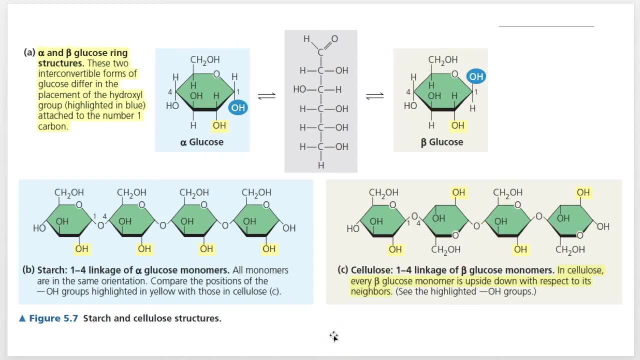 cellulose. so that is an indigestible fiber, right? so if you feel like, oh, i gotta eat wheaties because i need fiber or whatever i don't know, um, you gotta eat your leafy greens to get cellulose in your uh colon to help clear out your colon. that's what this is. so this is indigestible. 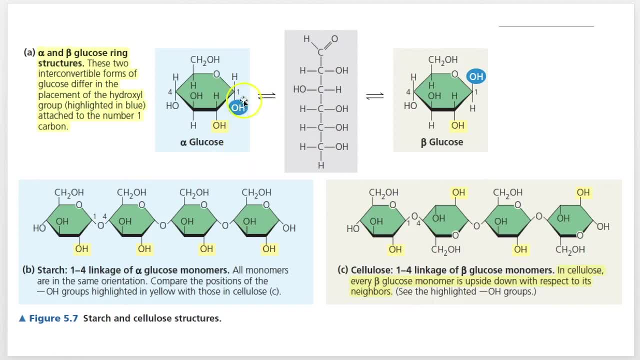 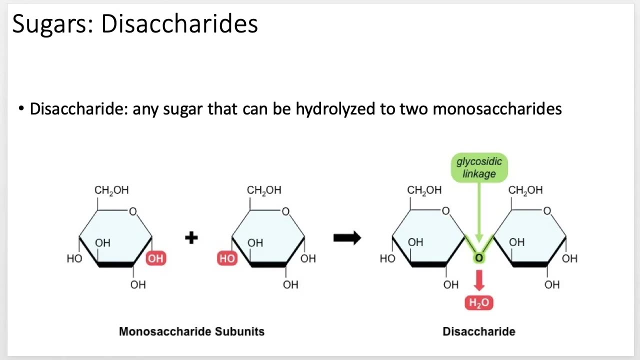 that one simple change. okay, so having that hydroxyl group, either point down or point up, can decide whether or not an enzyme is able to break it or not. really interesting. so that leads us into these types of linkages. which these types of linkages? let us form disaccharides, so that's. 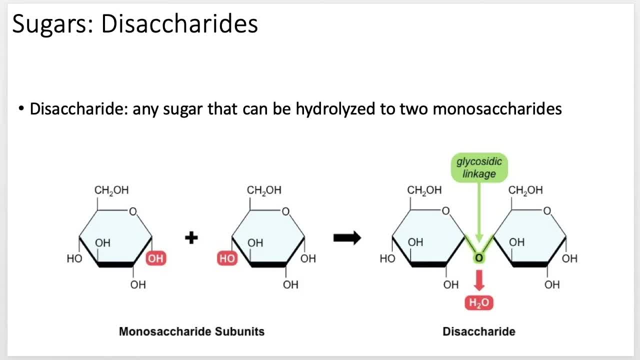 where we're going to take two monosaccharides- whatever they are- and stick them together using a glycosidic bond or a glycosidic linkage. it's just a dehydration reaction, okay, or yeah, infused there's condensation reactions and there's dehydration reactions, so dehydration reaction. 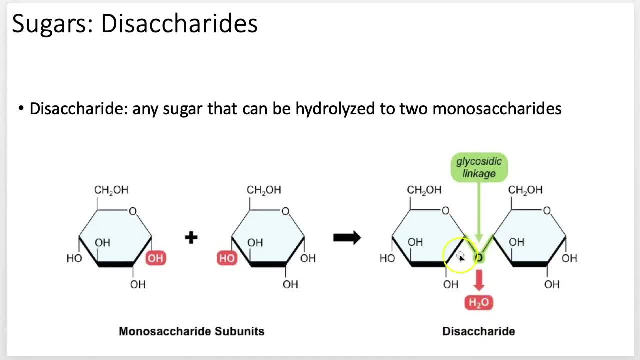 is the loss of water if during a condensation reaction- whereas a condensation reaction isn't necessarily a loss of water, it's just the loss of a small molecule- when you're combining two things. so dehydrations are condensations, but not all condensation reactions are dehydrations. 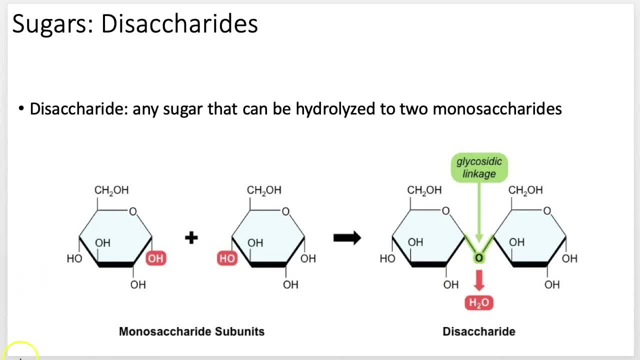 whatever you're forming a glycosidic linkage here between these two. now i wanted to go back to that original video that we were watching and they're going to talk about the different dissect rates that exist and the kind of foods that they're in. glucose is the most important member. 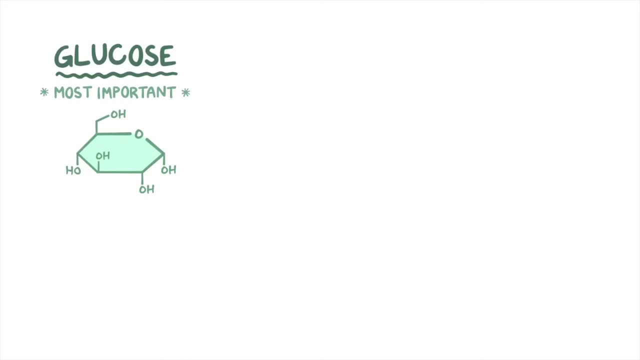 of the sugar family and it's a monosaccharide. it's one of the main sources of calories for the body and is able to cross the blood-brain barrier and nourish the brain. another monosaccharide is fructose, which is commonly found in honey, fruits and vegetables. 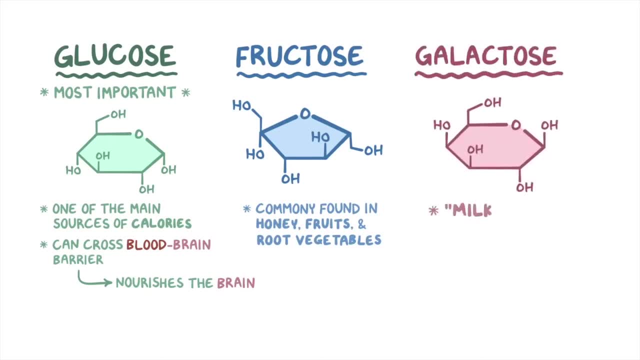 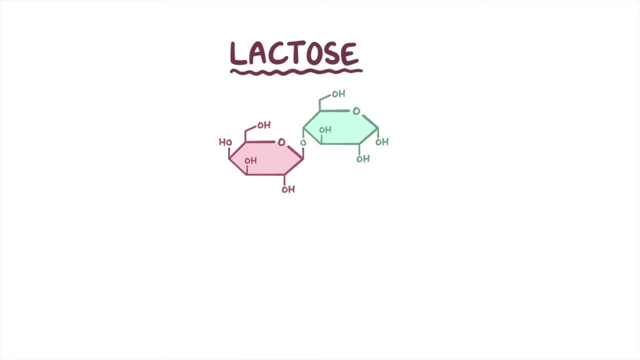 finally, there's the monosaccharide galactose, known as milk sugar. it's known as milk sugar because it's found in nature when it links with glucose to form lactose, a disaccharide found in the milk of mammals, which includes cow milk as well as human breast milk. sucrose or table sugar is another. 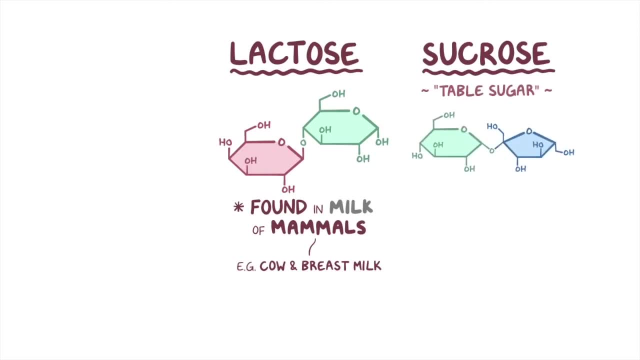 disaccharide, and it's formed when fructose links up with glucose. sucrose is found in various fruits and vegetables, with sugarcane and sugar beets having the highest quantities. maltose is another disaccharide- glucose molecules linked together- and it's found in molasses, which can be used as a substrate to 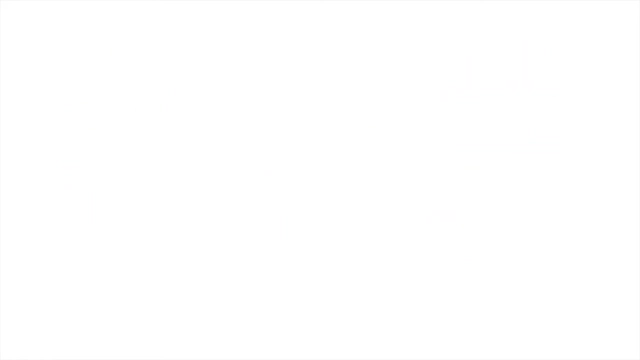 ferment beer. sugars like fructose, for example, are most always found in combination with other sugars, and the combinations can be pretty different, even in seemingly similar foods. for example, in honey, fifty percent of the sugar is fructose, forty-four percent is glucose, four percent is galactose and 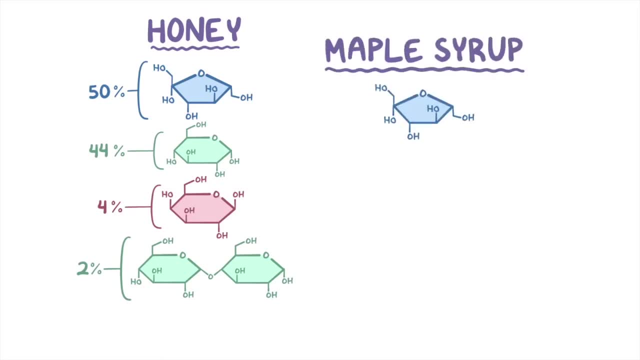 two percent is maltose. we're sitting here with two glucose molecules linked together, and it's found in molasses which can be used as a substrate to ferment beer maple syrup. less than one percent of the sugar is fructose, three percent is glucose and 96 percent is sucrose. 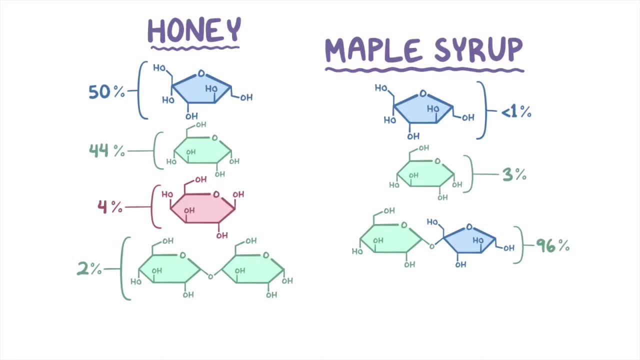 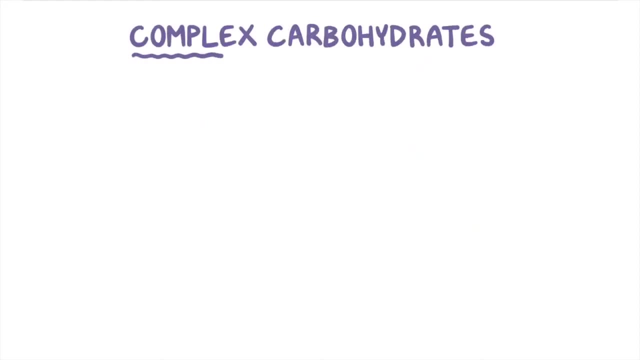 so simple sugars, whether they're natural or added, are mixtures of monosaccharides or disaccharides. next, there are the complex carbohydrates. there are oligosaccharides like galacto-oligosaccharides, which are short chains of galactose molecules like those found in soybeans. 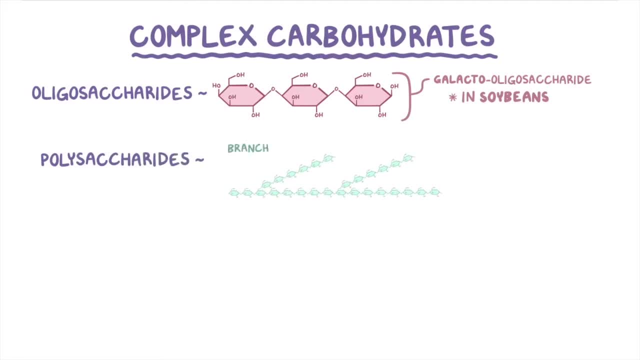 polysaccharides, which are even larger chains with branches and are the most abundant type of carbohydrates found in food. Starches are polysaccharides with molecular bonds between sugar molecules that human intestinal enzymes can break down. Starches are an important 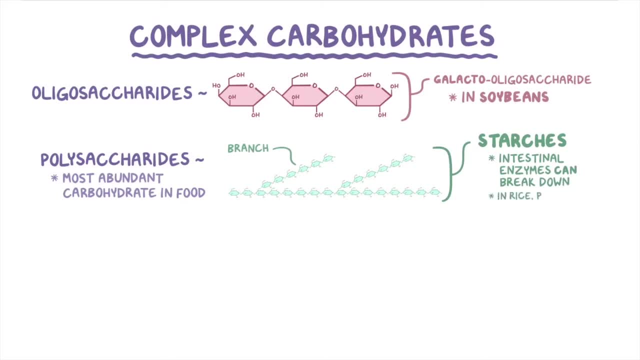 source of calories and can be found in foods like rice potatoes, wheat and maize Starches don't taste sweet like simple sugars because they don't activate the taste buds in the same way, And there are also dietary fibers, which are carbohydrates that intestinal enzymes 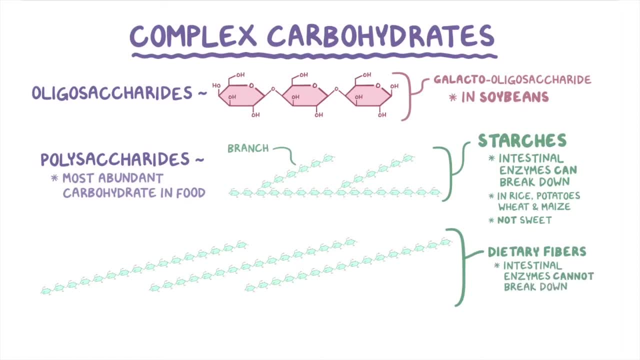 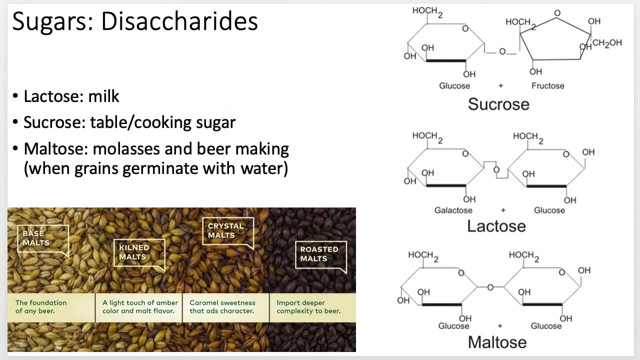 can't break down and so the body can't digest them. You'll probably start feeling the same after eating them, because they are full of fiber and fiberatanins and it's a little bit more of a mixture, but molasses is the big one. 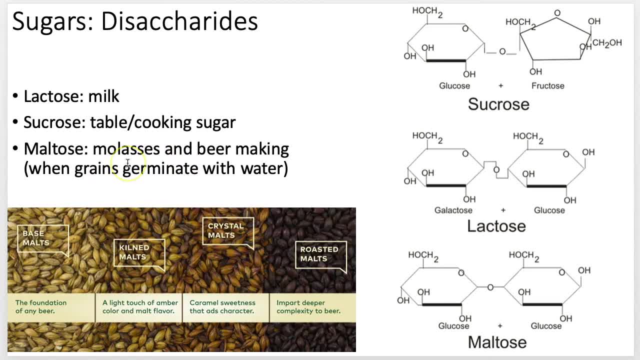 that you encounter that in, And if you're making beer, you germinate the. I live in Colorado where they make a lot of beer, So you get your malt and you germinate it in water and then you get maltos out of it, out of the endospore, I guess. Anyway, doesn't. 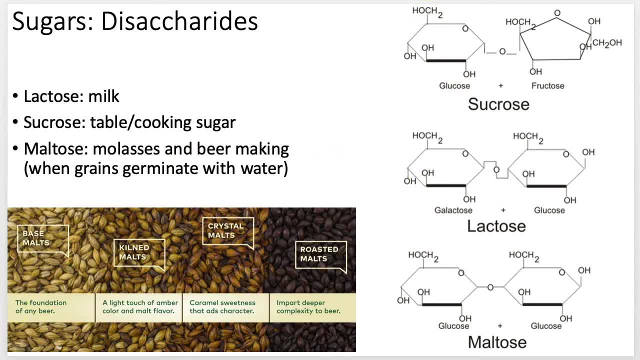 really matter. It's just the different combinations of your various monosaccharides. so that's and that's how you get your disaccharides Awesome. Now let's move on to a little more complicated. We're going to start tacking on more and more sugars And, as we start tacking on more. 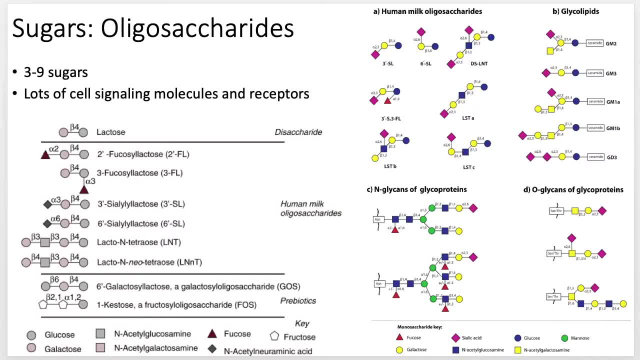 and more sugars. we call those oligosaccharides, So basically anything under 10 would be considered an oligosaccharide, though I'm sure you could find examples of oligosaccharides that exceed nine sugars, But for the most part most of our oligosaccharides stay under that boundary. 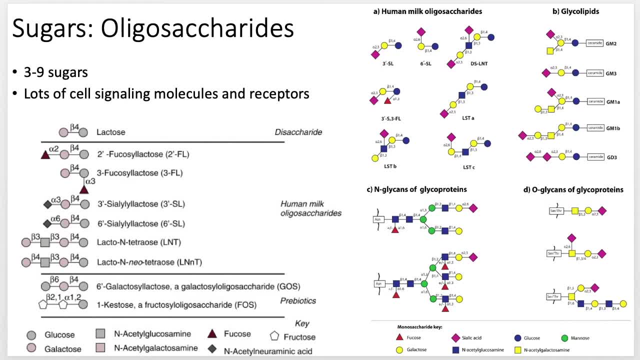 So if it's three, because it's a disaccharide, so the disaccharide is two, so we're going to move on to trisaccharides and beyond, And that's basically. it's not really for energy consumption. 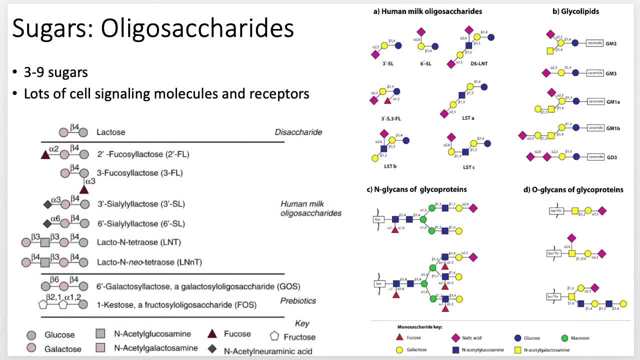 though you could break these sugars off and use them for energy, They're more for signaling. So tons of signaling molecules are oligosaccharides, by themselves or attached to proteins, And so just by themselves they can be signaling molecules. So here are just a bunch of examples. 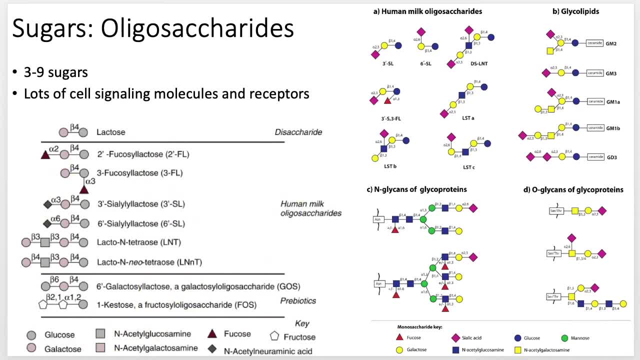 In human milk. prebiotics, which is something basically. a prebiotic is what bacteria can consume that are probiotics that then, like, make your health better. So you can eat prebiotics to make the probiotics work better. It's a whole subfield. that's mildly under my PhD, but I don't. 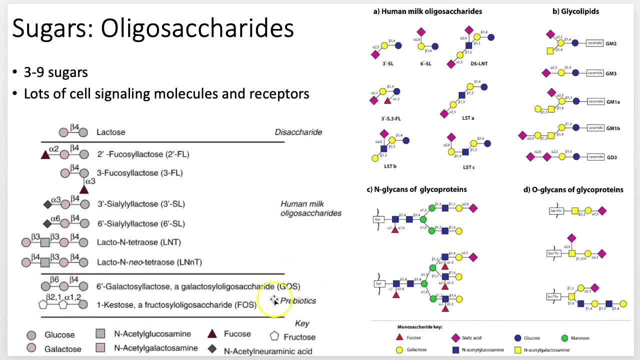 know we don't have to talk about that, But anyway, prebiotics are interesting. You should eat healthy food- is what this really means. Don't eat gross stuff because it's all artificial and all the sugars are artificial. You can see the variety. So I like these charts because they just if you get super into this. 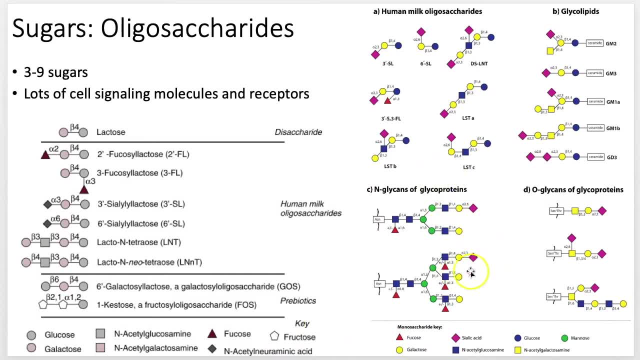 stuff. then you can just see: oh, this one's got a few ghosts on the end. Oh, wow, That's very interesting. Oh, and a galactose- Wow, That's very, very exciting. Anyway, you can see it gets. 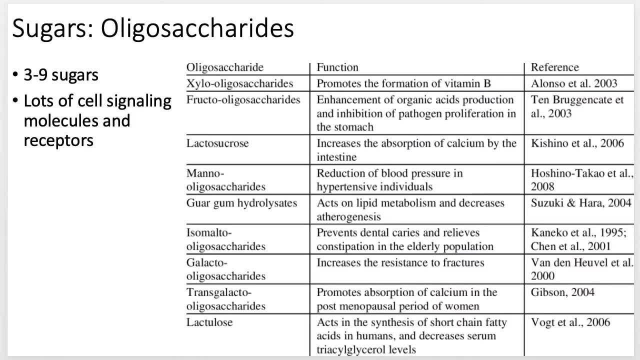 kind of complicated as you dig deeper. Some people are super into oligosaccharides, some people are not. It doesn't really matter, but they do have a wide variety of associated functions, guys. So from vitamin B to blood pressure changes to. 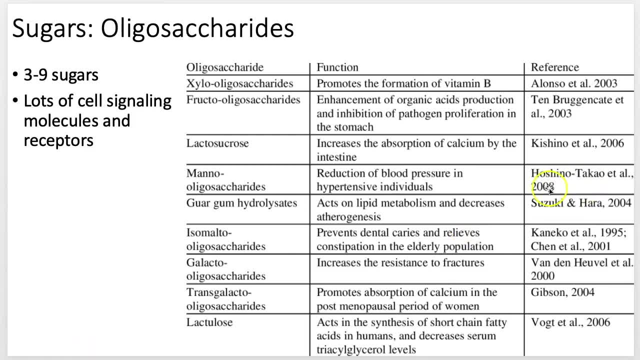 you know, absorption of calcium and menopausal women. like it's crazy. I clearly got this chart from an older paper because these are all from like when I was in high school, But just to give you some idea of the variety of functions that these really big oligosaccharides can have Now. 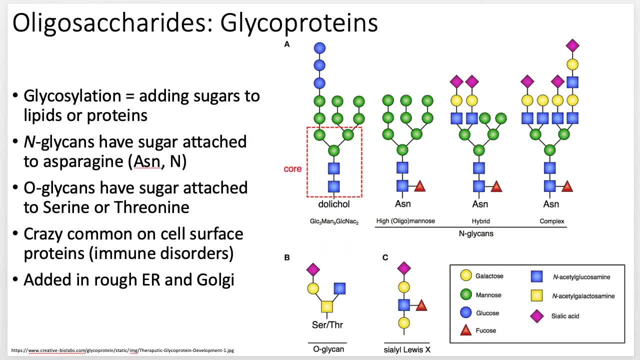 jumping off of that. they don't have to just exist by themselves. We can take oligosaccharides and attach them to proteins, specific protein residues, and we can then have them serve a function. So they can be a cell surface receptor for something or they can be a cell surface marker to mark a cell. 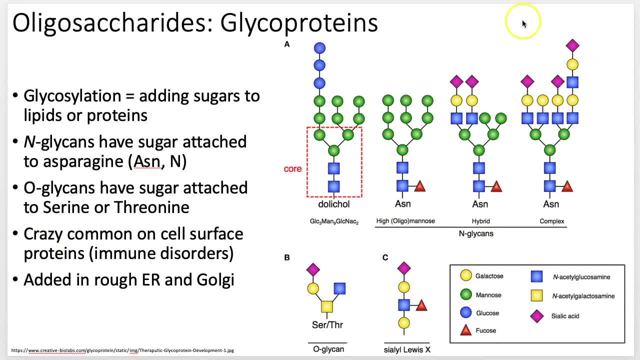 for whatever. There's so much variety that you can actually engender in these that it gets incredibly complicated, really, really, really, really, really fast. Okay, Now there are two types. We call these glycans, So that's glycoproteins when we glycosylate. Okay, So glyco meaning like sugar. 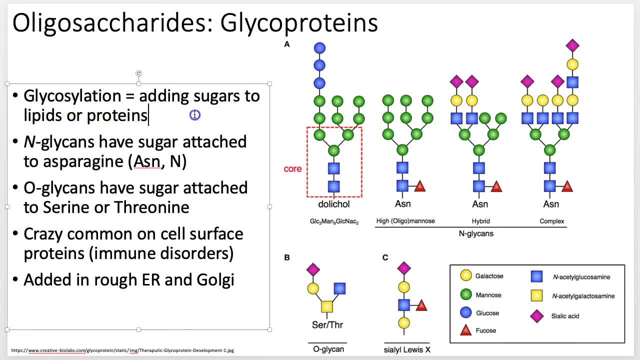 and salation, basically meaning we are attaching- So that's when we're attaching sugars- to either lipids or proteins- Okay, And I'll show you some examples of lipids too, But for in this case we've got like asparagine. 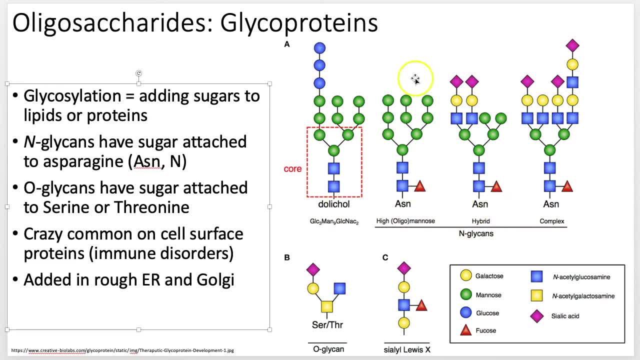 down here right, Which is our, an amino acid, And so we're going to take some sugars and attach those. So we're going to take our oligosaccharide, our multi-sugar chain, and we're going to attach. 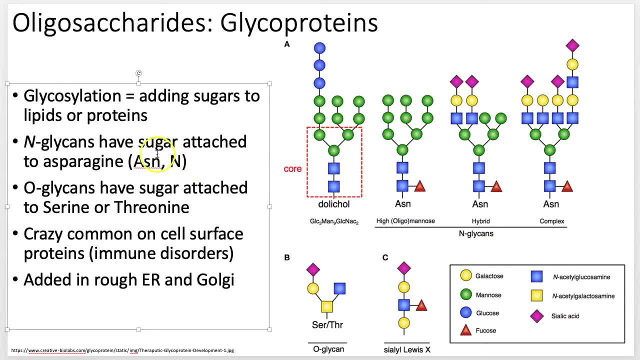 it to either an asparagine- Okay, So that's called an N-glycan, Okay- Or we can have O-glycans, which that's where you attach it either to a serine or a threonine, Okay. 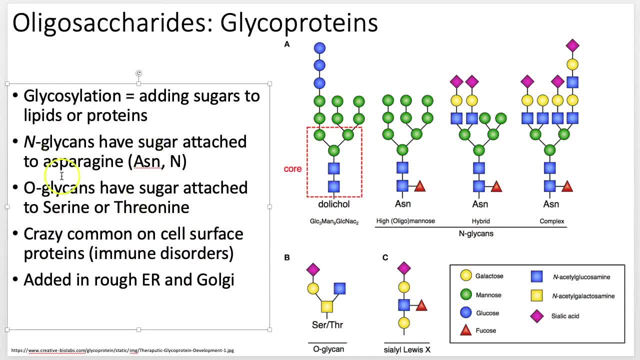 This is me being crazy, Crazy common on cell surface proteins. Yes, You can have immune disorders where you are not properly either putting these on or they're you're putting the wrong ones on the cell and that can cause an immune disorder because we use these to. 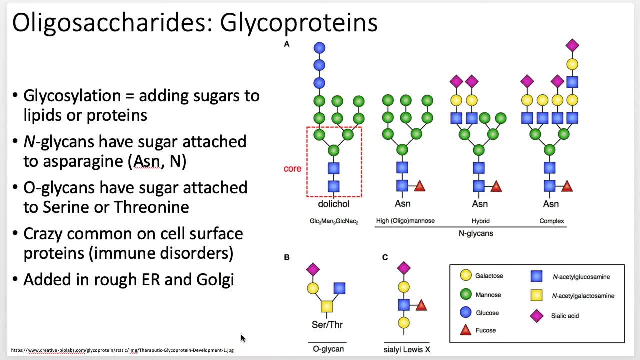 recognize cells for their functionality, Like, oh, is that a T helper cell or not? Well, that's a good question. Let's look at it. Let's look at their proteins and see if they have the correct oligosaccharides, And so it's really interesting. So they're added on in the 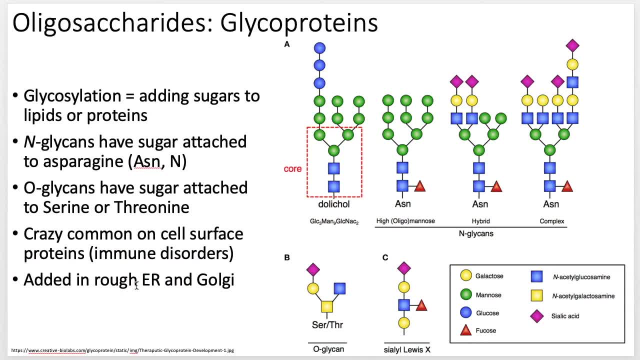 rough endoplasmic reticulum because it's a protein right. That's usually that's going to be put on the surface of a cell. So that has to go through the rough ER and that's where you get your initial addition. And then it's going to go to the Golgi to have extra polysaccharides added. 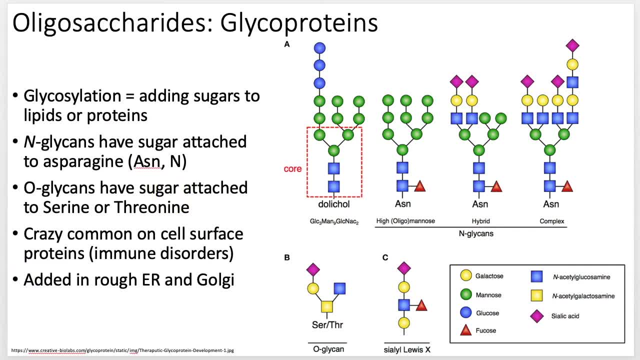 or extra saccharides, Sorry. So there's a video that I want to show you. I apologize for the quality. It's like the best version of this video I can find, And it drives me crazy because I'm like, oh my gosh, this video is super good. The quality is like really bad, but the content is. 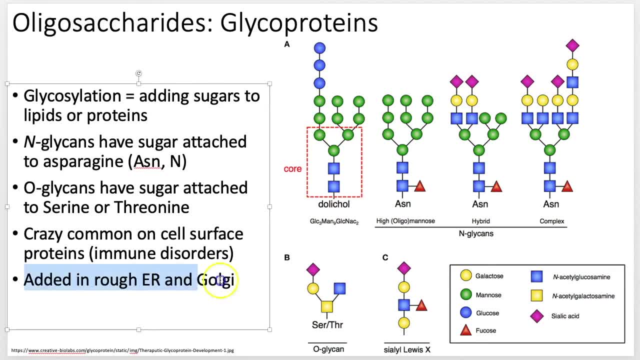 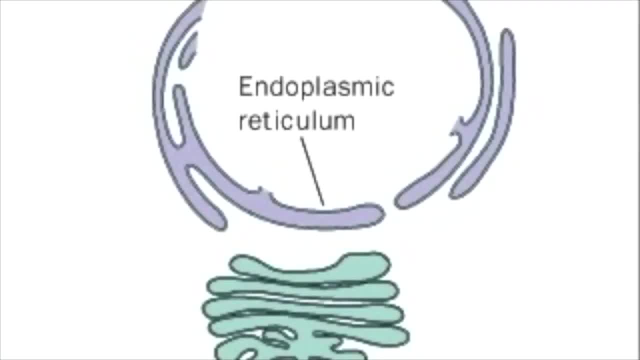 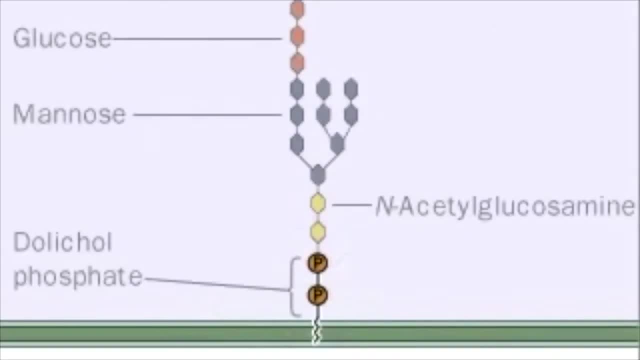 so good, So we're going to cut to that. It's going to show you this process. actually, Glycosylation- adding sugars to proteins- begins in the endoplasmic reticulum and continues in the Golgi apparatus. Let's examine the process for one. protein Enzymes in the ER remove glucose. 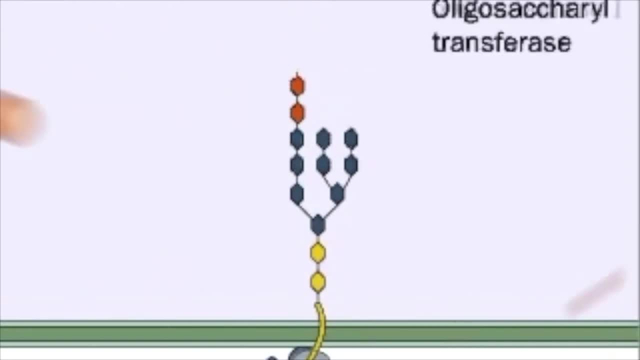 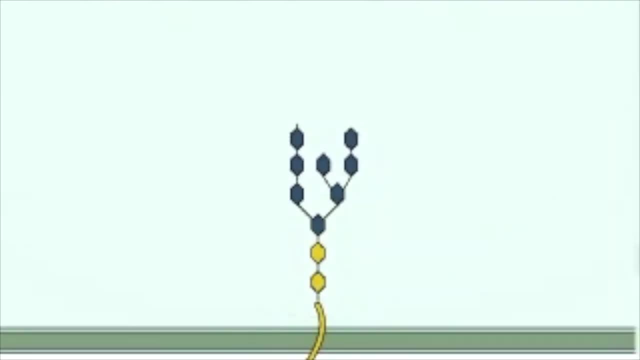 and mannose residues from the oligosaccharide chains. Vesicles transport the glycoprotein to the cis-Golgi network, Where one of two events occurs: Either N-acetylglucosamines attach to the oligosaccharide. 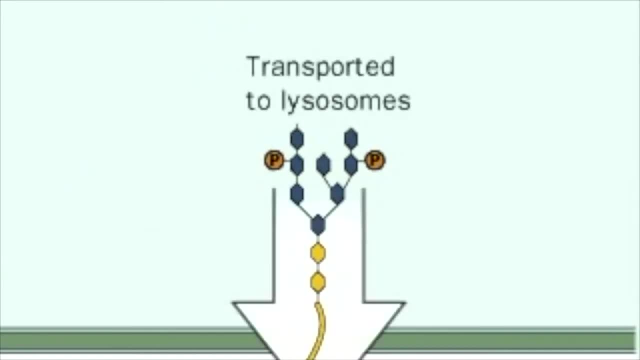 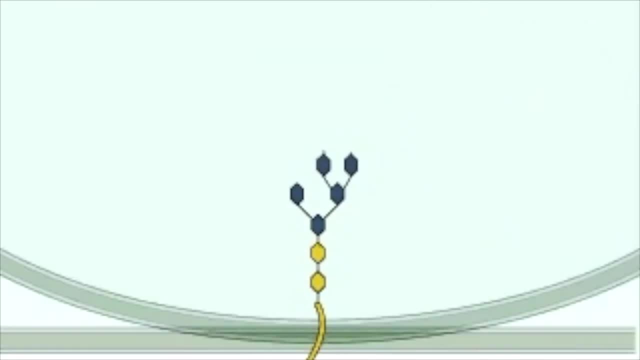 and are transported to the lysosomes Or enzymes, remove more mannose residues. Vesicles transport the modified glycoprotein to the medial Golgi cisternae, where N-acetylglucosamine attaches and more mannose molecules leave the molecule. 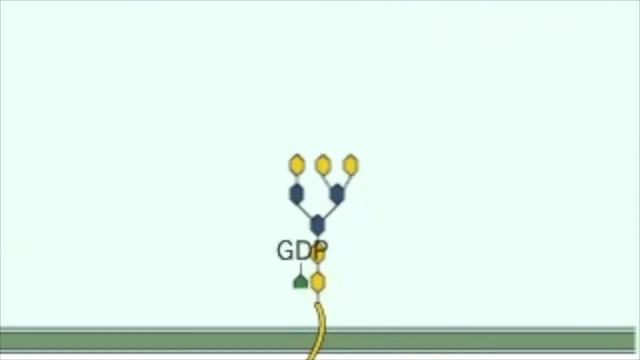 Vesicles now transport the glycoprotein to the trans-Golgi cisternae, There galactose and sialic acid join the chain. The glycoprotein is finally ready for transport to the cis-Golgi cisternae. 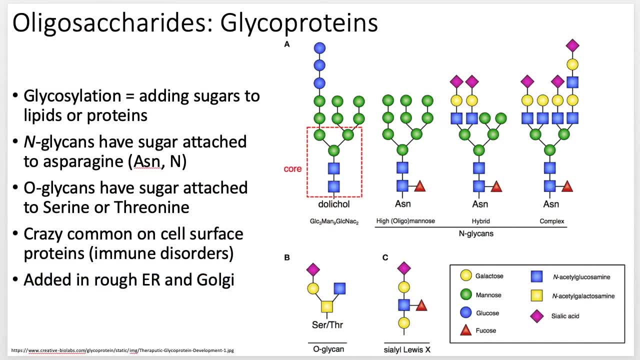 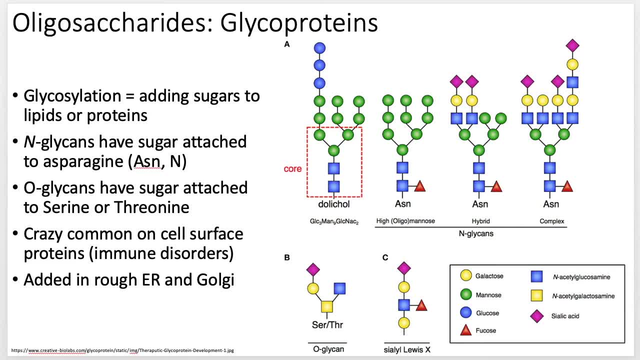 I have emails, св. I have emails that explain it very well and have the amount of miles it takes to do it. So, yeah, I hope, don't follow me too much. I hope it helpful to you Everyone. as always throughout this program, we will try our best to help you. 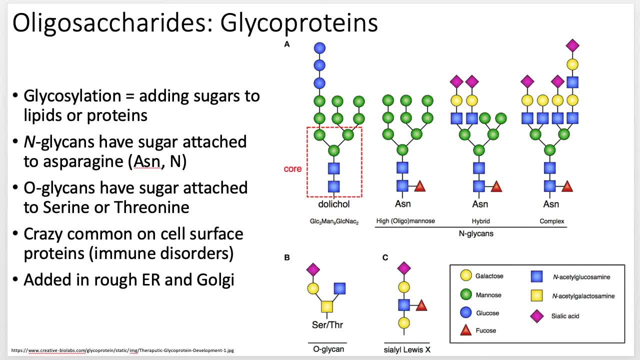 Hopefully we will answer all your questions daily, As always. 촬영 of these sugars on proteins, And so this is going to come from a pharmaceutical company that sells reagents to actually do this kind of work. Secretory and membrane proteins are often. 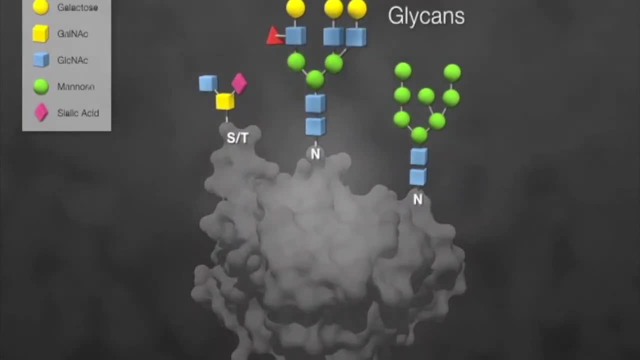 post-translationally modified with sugar chains called glycans. Glycans are essential for the stability and function of the mature protein. They affect enzymatic activity, half-life and receptor binding, among other biological processes. Proteins can be modified with. 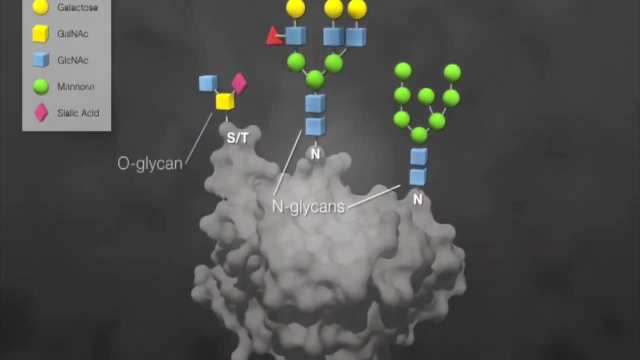 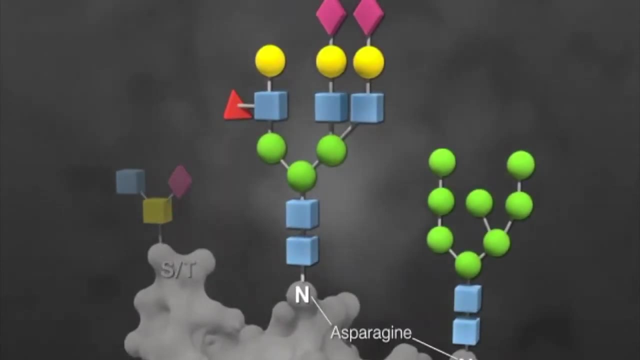 different kinds of carbohydrates, N-glycans and O-glycans being the most common types in eukaryotic systems. N-glycans are attached to asparagine residues of the protein shown with an N. N-glycans have a common biosynthesis pathway, which is reflected in 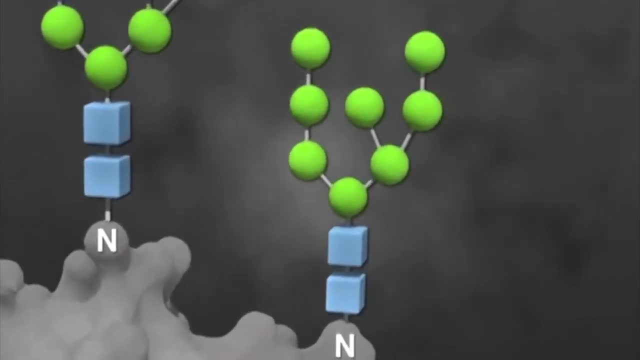 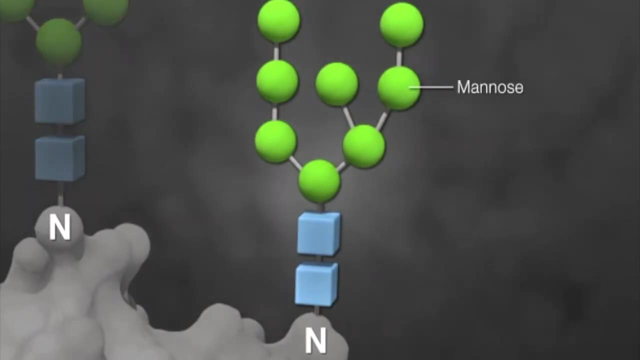 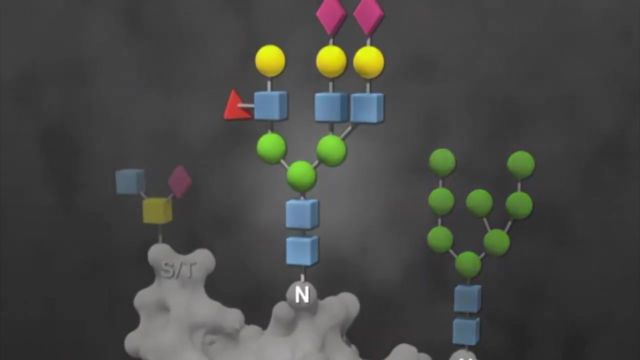 the common structure of their core. N-glycans can be high mannose, which means all the components monosaccharides are mannose residues, with the exception of the two-core N-acetylglucosamine or glicknack residues. N-glycans can also be complex, which means the mannose residues are. 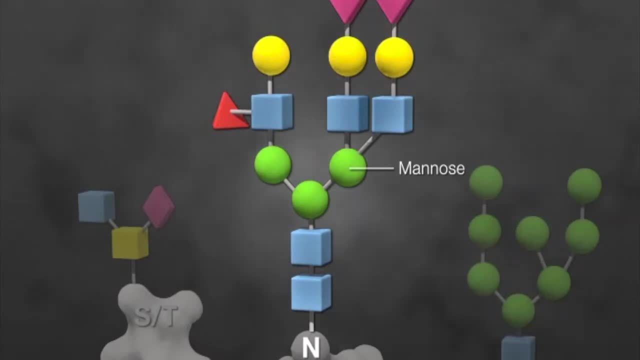 only present at the core and the branches are extended with other monosaccharides such as N-acetylglucosamine or glicknack. galactose, sialic acid and fucose O-glycans start with the addition of an N-acetylglycosamine. 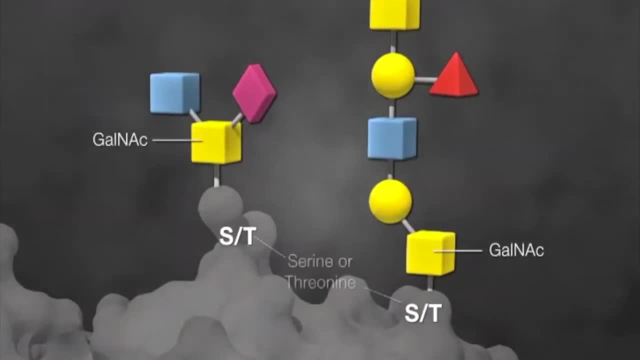 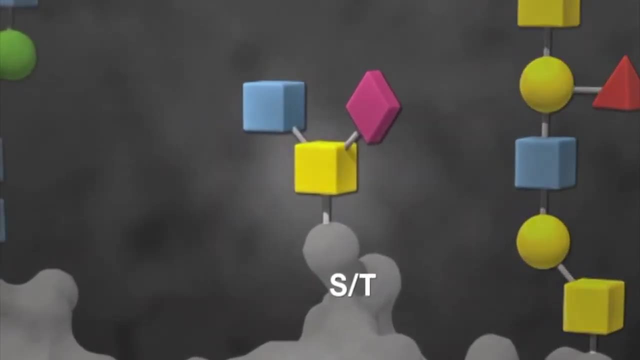 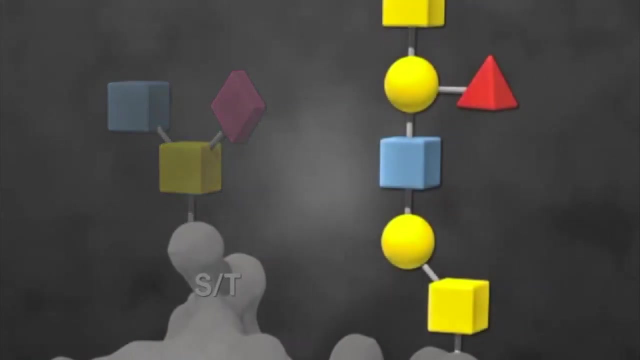 or galnack residue to a serine, shown with an S, or threonine, shown with a T. O-glycans are often short chains consisting of only a few sugars, or they can be extended by the addition of different monosaccharides, resulting in a longer. 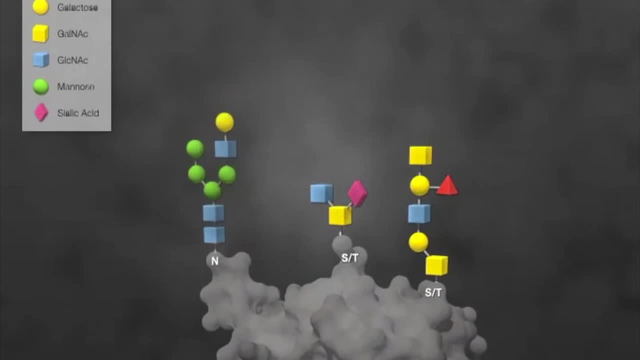 chain D-glycosylation refers to the removal of glycans from proteins. Enzymatic D-glycosylation is the method of choice because it preserves the integrity of the protein. N-glycosylation is the method of choice because it preserves the 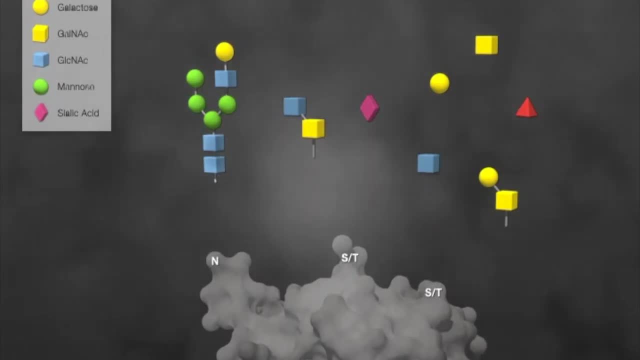 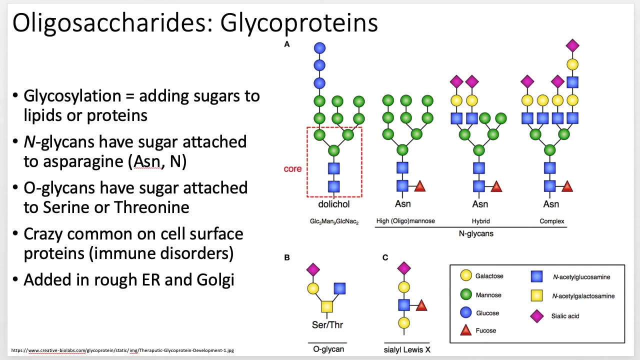 integrity of the protein and sometimes the glycan chains for further analysis. A much higher quality video from New England Biolabs- or NEB as we usually call it if you're a nerd- And they basically sell the reagents and the equipment to analyze the oligosaccharides on. 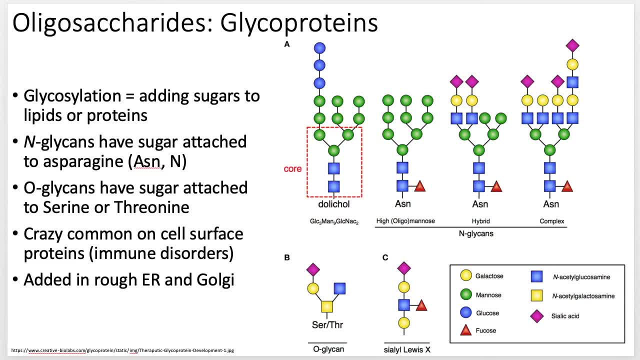 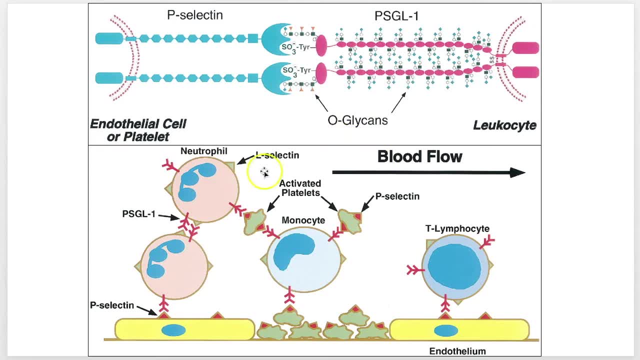 the surfaces of cells. And those are just ways that you can study a cell and see what it's trying to do. So where else do we see oligosaccharides? So you know there's a lot of different ways to study oligosaccharides. So here is an immune example. So up here we have. 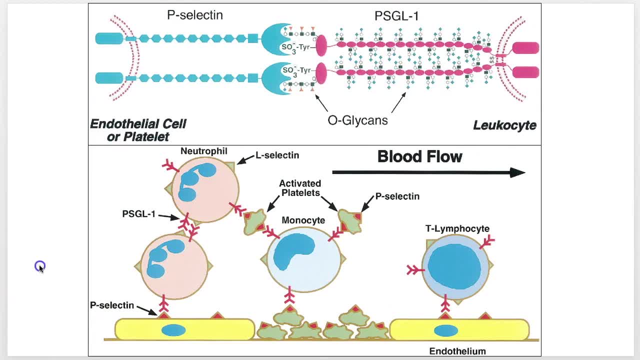 P, selecum and PSGL1.. So it turns out that immune cells like to travel along your blood vessel. So this is the blood vessel. There's a blood vessel wall that your endothelial cells and your immune cells. So here we got some neutrophils and some macrophages or monocytes. 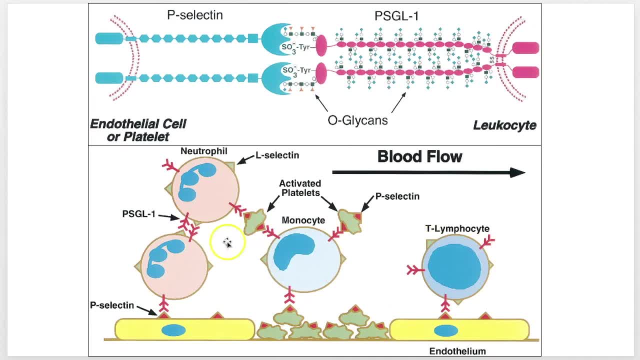 when they're flowing in the blood. but they're macrophages And there's a T helper cell And all these guys will express PSGL1, based on the actual presence of cytokines that are in the blood. So they're floating in the blood And so if they're expressing that, they kind of reach out with. 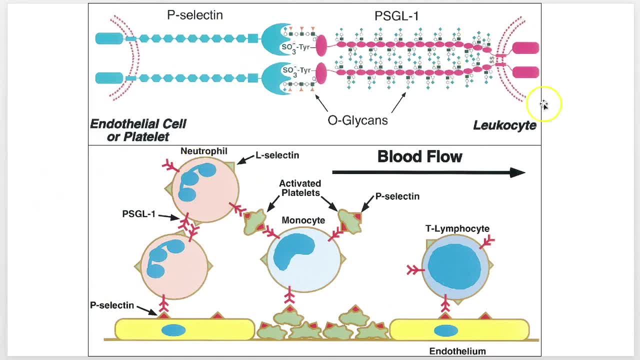 little grabby arms and are looking for this molecule. So the leukocyte or the neutrophil T cell, whatever it is, is reaching out with this PSGL1, which is covered with all these sugars, And those sugars need to match up with P selectin, which P selectin is expressed on the 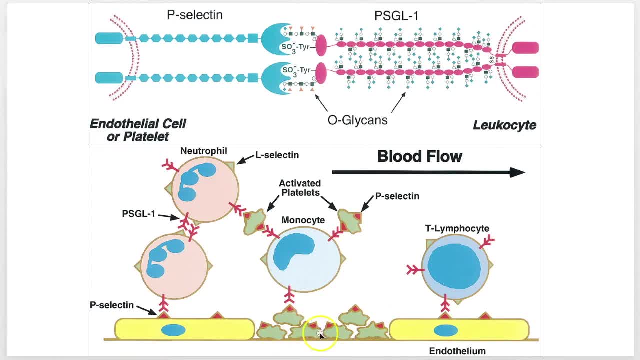 endothelium, And so you can imagine, let's say, down below, where my cursor is, down here. So down here I actually have a like. somewhere there's damage, So maybe there is an invader. I've got a cut going on And so you can see I filled the cut in with platelets here, but I'm 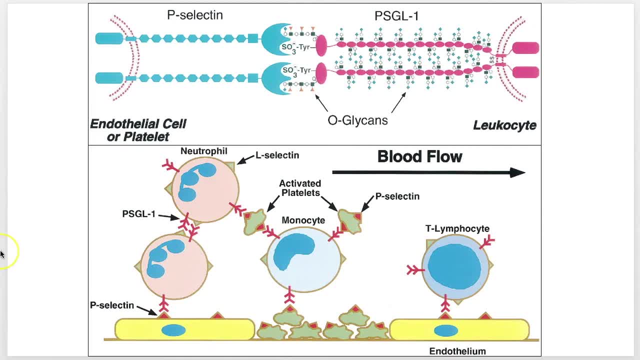 going to express P selectin nearby to reach out and grab the little arms of the PSGL1s from the immune cells, And so they only recognize those because they are glycosylated properly, which is really, really interesting, And bring it back to immunology. So glycosylation isn't relegated just 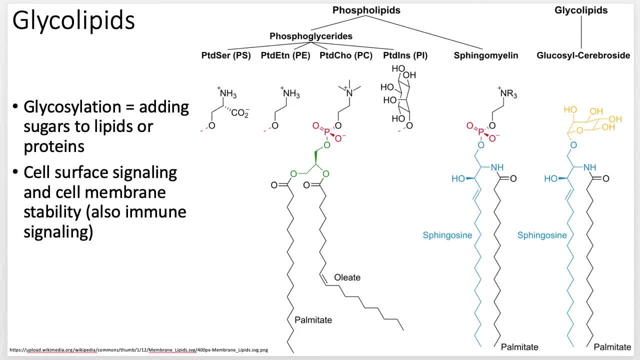 to proteins, though You can also glycosylate lipids. We call those glycolipids. Okay, If I attach some kind of sugar to it? okay, those are glycolipids. There's a huge variety of these. 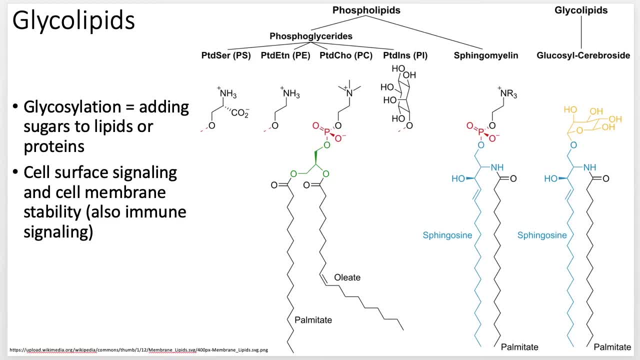 just like there are glycoproteins. Just having them on the cell surface can signal things, but oftentimes you can also put them into the cell membrane. It can either add to stability, it can detract from membrane stability. It just kind of depends on what you're trying to do And 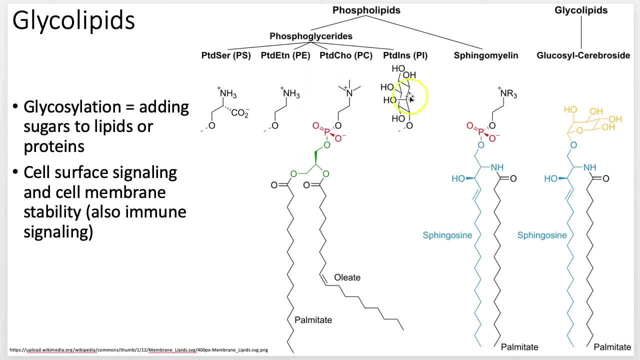 it has more to do with this end of the structure is where we're actually adding. So this is the only glycolipid on here, is this one. It's just to contrast it with these other guys. but you could put it on the on the surface here and that could signal to another cell, because this is what would 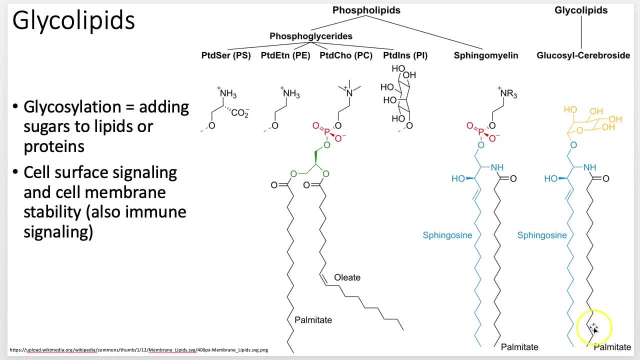 be facing out right And this would be facing in towards the actual fossil of the bilayer, And so you can attach different sugars here and it acts as a signaling molecule. Now you could embed a protein and put sugars on it too, Like that's what we're doing here, But this is different, So you 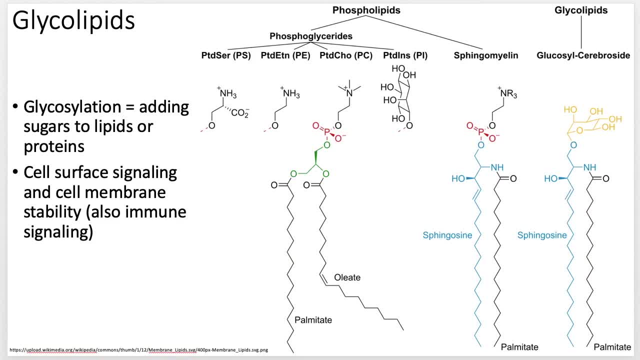 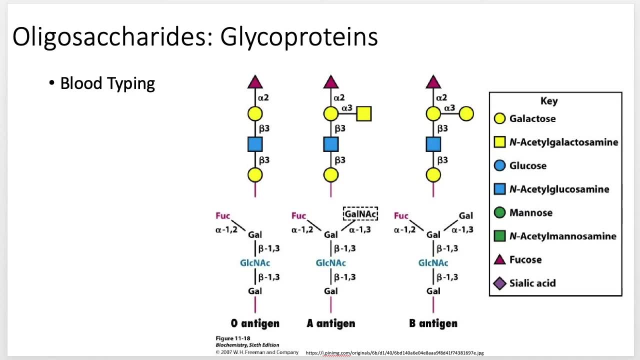 can just attach it right onto the lipid, which is kind of fun. Now another common example: blood type gets brought up all the time, But we need to talk about it because blood typing actually is based on glycoproteins and glycosylation of proteins. And so if you're O like, 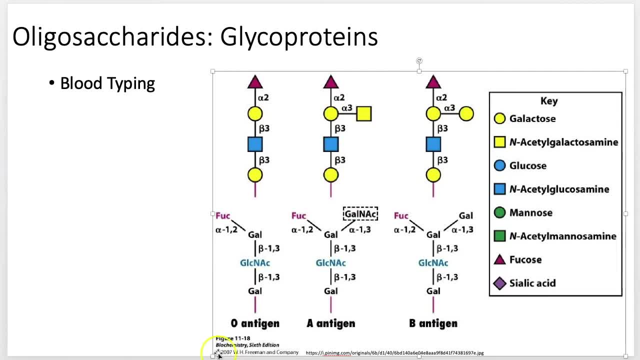 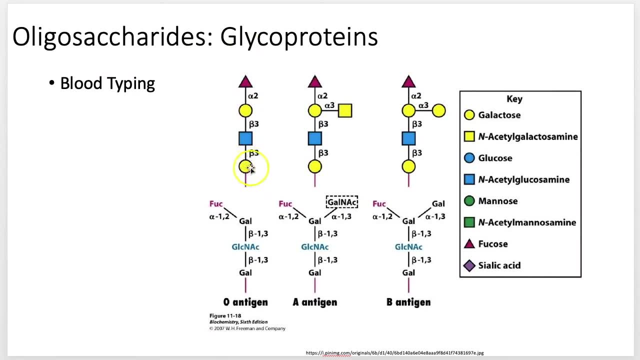 me. this is what the structure looks like, And I apologize for the quality- It's because it's like a 2007 picture, But so this is the actual structure. So you've got your galactose, you've got your N-acetylglucosamine, which is basically a glucose derivative with an 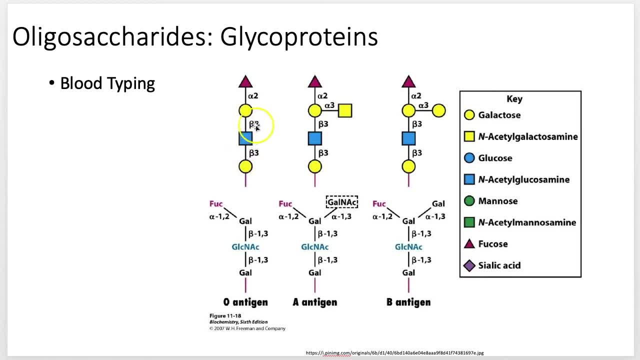 antigen, a nitrogen attached, sorry. And then you've got your galactose, and then you've got your fucose, And so you can see that that same structure is in the A antigen as well as the B antigen, And so that is maintained. And so the only real difference between A antigens is that 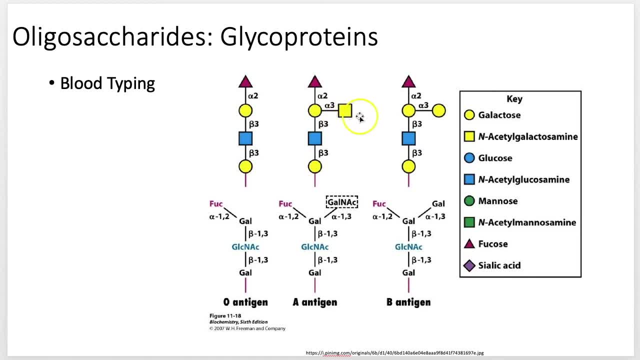 I tack on another N-acetylglucosamine or, I'm sorry, an N-acetylgalactosamine, Oh man, Or I replace that with a galactosamine, And so that's the structure, And then you've got your galactose. 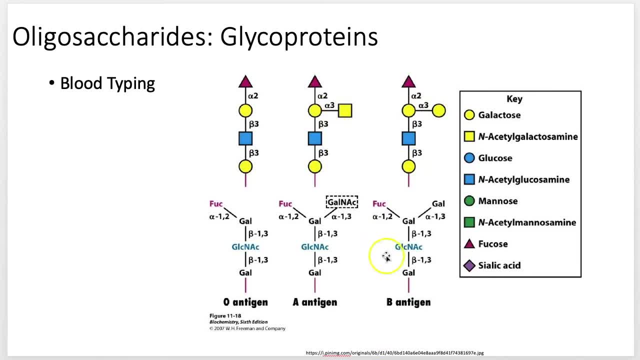 and you can actually express both of these. Okay, So if you were A B, that means your cells are co-dominant, They are expressing both of these. So you would have. if you looked at one of your red blood cells, it would have an A antigen sticking on there And you could look at other. 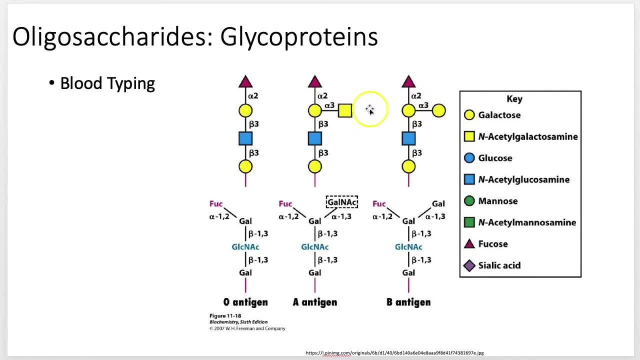 ones and they would have a B antigen on there. And that's the only difference. is this little square and this little circle Okay, But they all have the O possibility, Okay. So that's why O is the universal donor, because they can go into any of these cells and they won't attach, they won't. 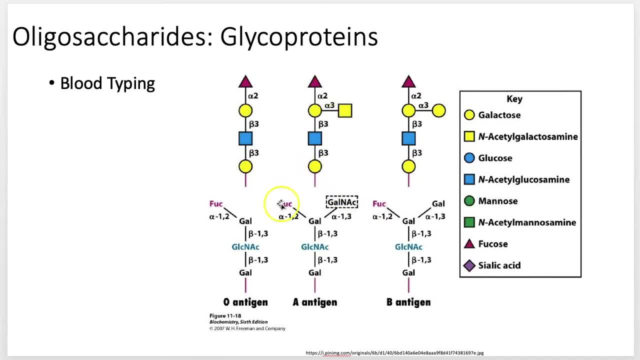 hack O as being foreign, because they all contain the O antigen. So the O is just kind of like subtly hiding underneath the A antigen and the B antigen. So this is why you can't take an A antigen and put it into an O patient. Okay, A blood and O blood don't mix, Um, but an A patient can take. 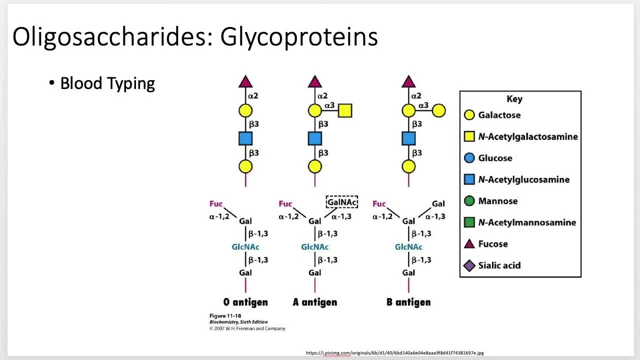 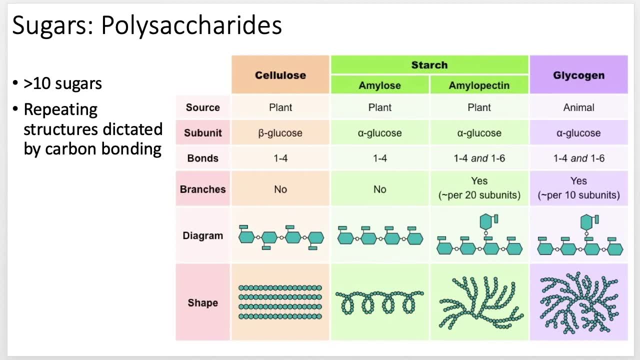 O, blood, Okay, And so that's where that comes from. Hey, I brought it back to the immune system again. Now let's get to some of the fun stuff. Let's talk some polysaccharides. So if you have 10 or more, obviously that's a caveat. So it's basically more 10 or more repeatable. So if you're 10 or more, obviously that's a caveat. So it's basically more 10 or more repeatable. So if you're 10 or more, obviously that's a caveat. So it's basically more 10 or more repeatable. So if you're. 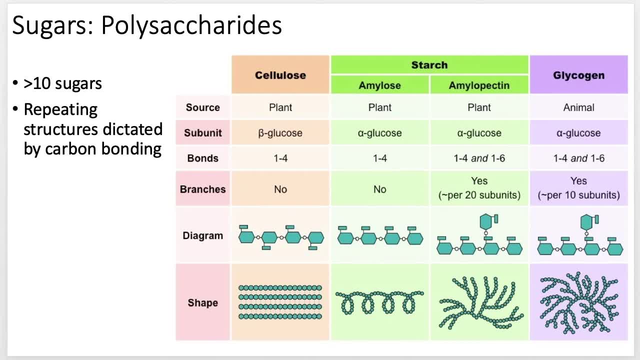 10 or more repeating units. Um, so that's contrasted with. I mean, obviously some of some of these structures can have more than nine. Uh, but for the most part, what we're saying is: okay, we have this continuous repeating unit, That's your polysaccharide. So, yes, they are. 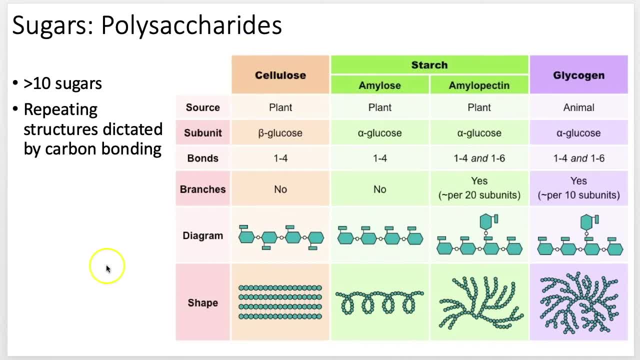 polymers, Um, but yeah, they're polysaccharides, And so there's lots of different examples: Um, cellulose being like the indigestible component of plants. Uh, it's like your fiber when you eat fiber. and then there's lots of other things, So different kinds of starches that you 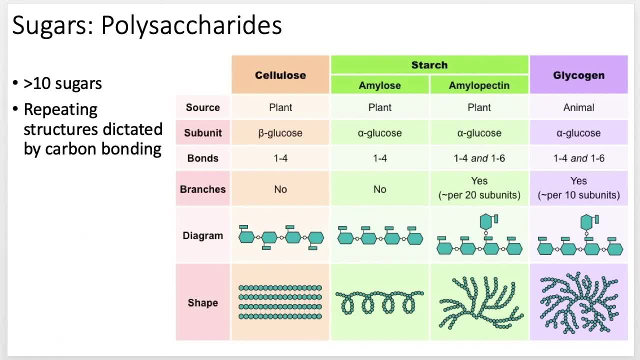 can eat, Um. and then there's polysaccharides, So different kinds of starches that you can eat, Um, and glycogen is what we use to store uh energy inside of our livers. Okay, We take glucose. 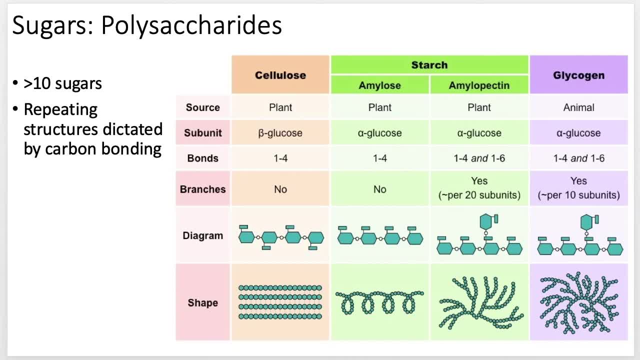 and we convert it into glycogen And that's just a longer term storage molecule. Uh, you're basically: uh, it's more efficient because you can cram more of it into a smaller space. Uh, and it's, it's. uh, it lasts longer, It doesn't get digested as rapidly, And so you can store it for long. Uh, 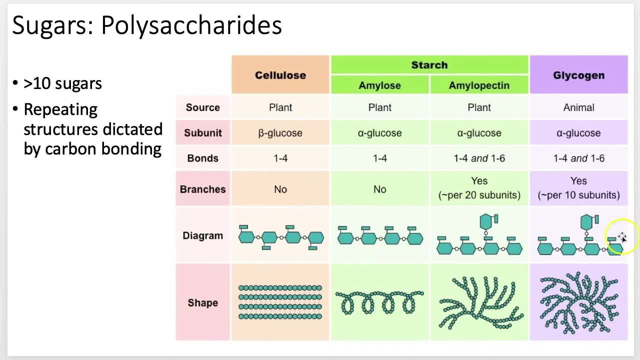 anyway, uh, branching is important, So how branched it is, uh, controls, uh, sort of how accessible it is, um, which is interesting, And uh, the actual structure of cellulose is really, really interesting. Uh, and so how they are organized, how we actually form those glycosidic bonds, is 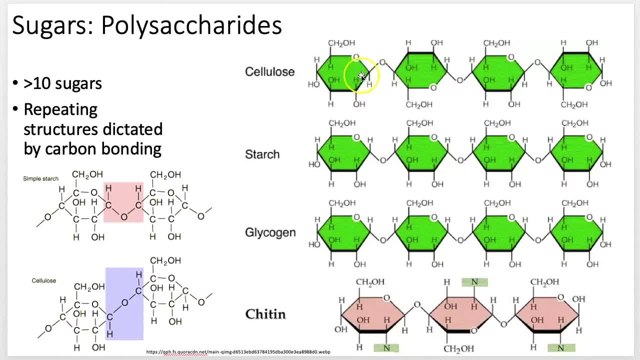 really really important. Okay, So there we have our, our beta glucoses. uh, where we're? we're flipping them, Okay. And then the starches and the alphas: um, glycogen and starch, notice, are really not that different. Um, and then, uh, chitin, okay, is where you're using an. 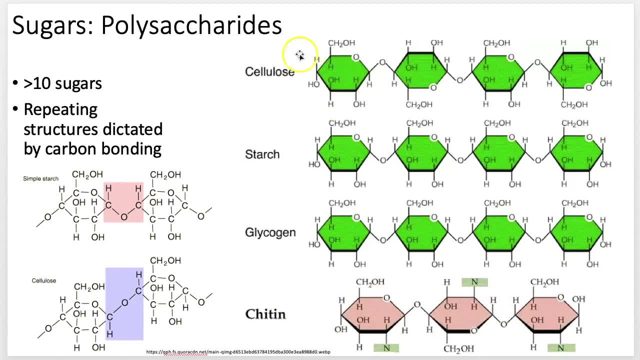 N-acetylglucosamine, in almost the exact same structure as cellulose. So you see, you get that structure. structurality, that's not the right word- the uh, the power of the structure, uh, because you have this bond all going up and down. So you get the. I don't know. 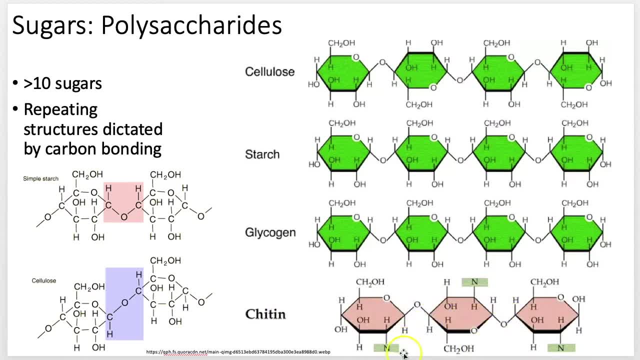 the structural power of it. Uh, but it's just a different sugar molecule because we took an N. let's take an N on there instead of a hydroxyl, Uh, but it's still. the structure is very, very, very similar, right? So that's polymers, Other polymers. So, uh, if you've taken a, 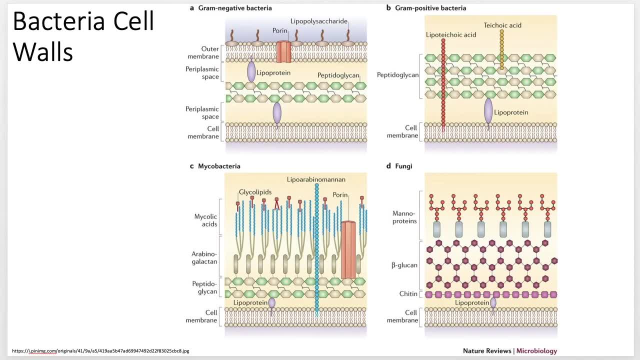 microbiology class. you may know that, uh, peptidoglycan, uh is a really important component of basically all bacterial cell walls, Um, and so you can see it here in the brown and green alternating. So that's the, the glycan portion. Uh, the peptido portion is the little. 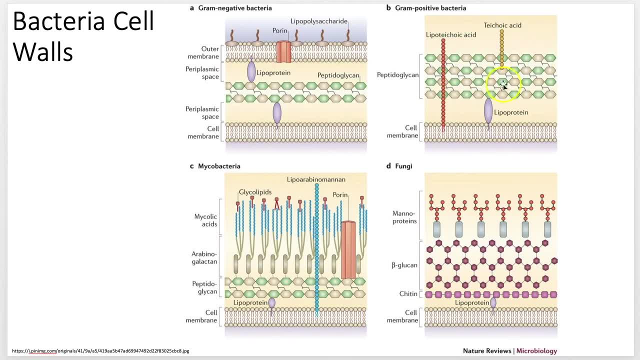 amino acids that are connecting them together here. Okay, So gram-positive bacteria have a huge, massive, thick chunk of peptidoglycan. Gram-negatives have a nice thin layer. Uh, mycobacteria also do have peptidoglycan. Um, it's not as easy to kill them though. 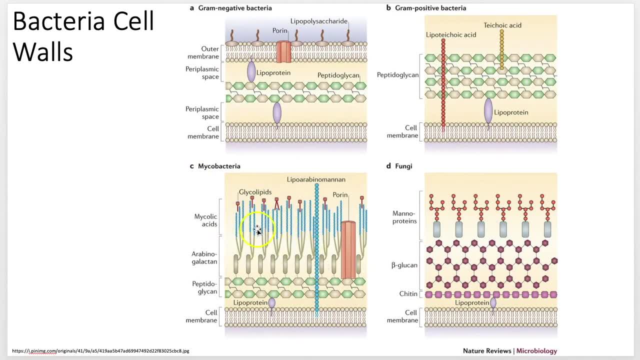 because they have this giant massive set of glycolipids. Hey, look at that. So we've got our uh, our lipid portion, Uh, and then we're going to stick on a uh oh, I guess this is the lipid portion. And then you've got the little uh glucose or whatever it is. I 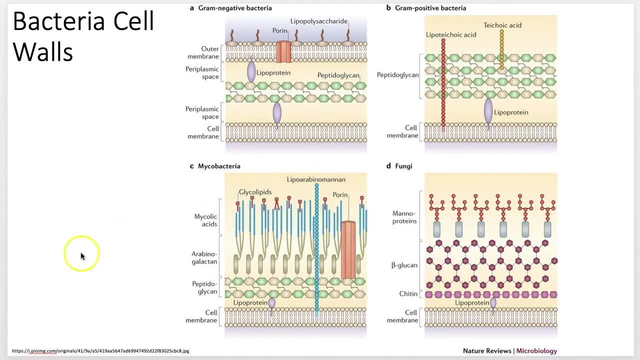 don't actually know which is, uh, mycolic acid, Uh, but anyway, so you can see, you're able to glycosylate and that's really, really important for structure. And over here on funguses which also have chitin as a structural component, um, there's other things too. So, uh, you've got. 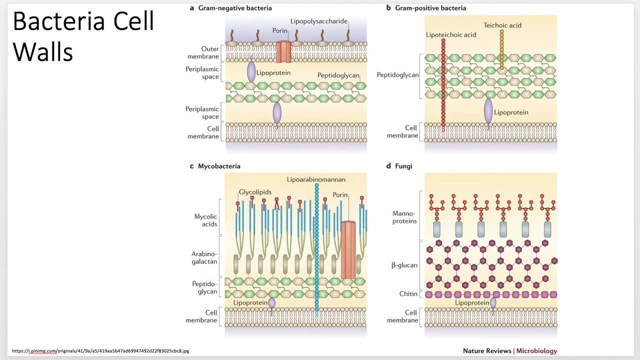 proteins with a bunch of mannoses on them, You've got beta-glucans, Uh, so you can see, it's not just glycosylate, but it's also glycosylate as well. Couple of things I wanted to talk about. Uh, I. 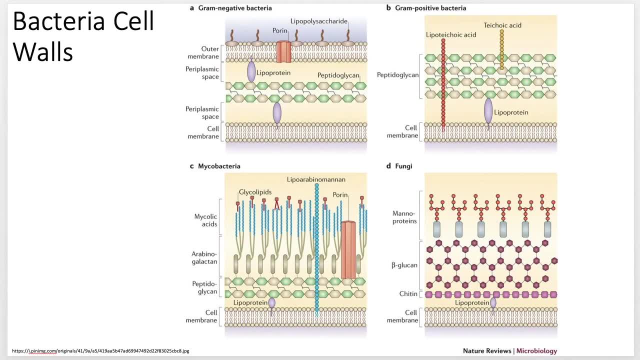 want to give you some actual examples. So, um, because, let's be honest, I struggle with keeping carbs interesting, I mean, I've tried to give you some examples where, like signaling molecules or whatever, like you can dig really deep. Um, but uh, a couple examples that come out of things. 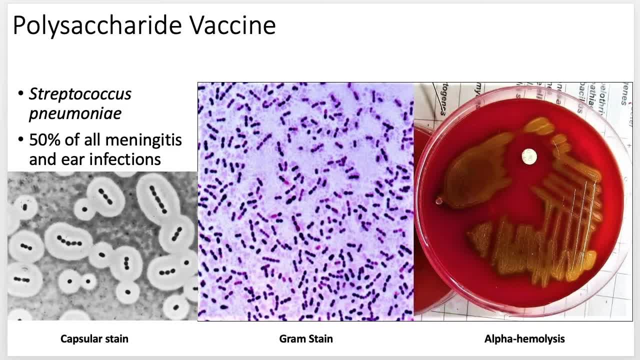 that I'm interested in. So vaccines I've always been interested in, And so, uh, there's actually a polysaccharide vaccine that we have. Uh, there's actually two types of them, And they're for for strep pneumonia. So the trick with strep pneumonia, which causes, like so many diseases, 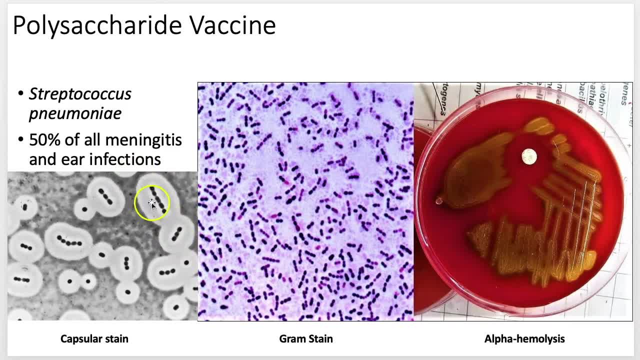 it's really bad. Uh, so it's streptococcus, right, So it's a string, a little string of cocci, little little circles, and they have a really powerful capsule. uh, powerful meaning, it's like a really 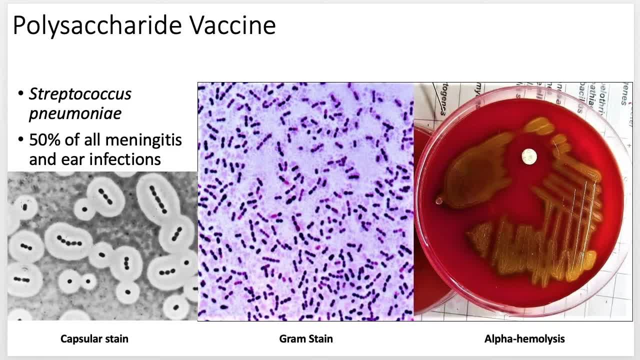 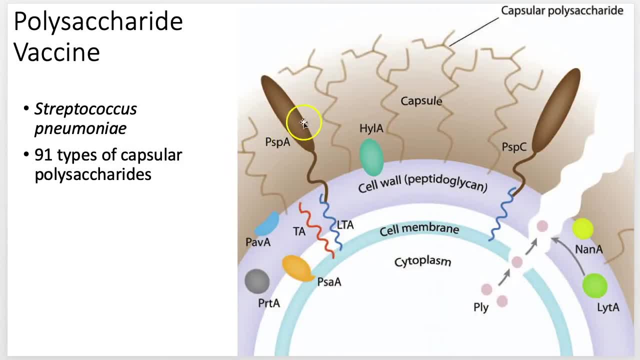 strong virulence factor. So, uh, that capsule, uh, of all these mucusy, sugary looking things, uh prevents uh immune cells from attacking it. And so, uh, here is the. there's the bacteria itself, right. So there's, it's a circle, right, It's a little circle, right, It's a little circle. 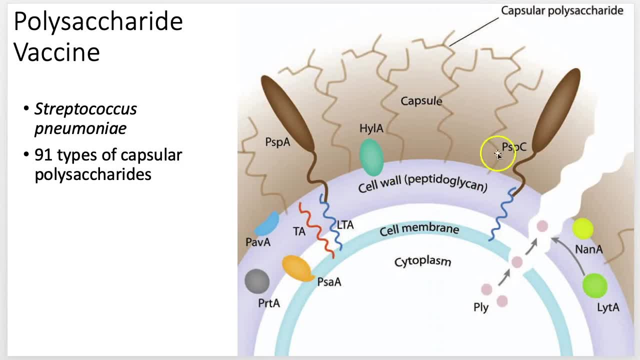 Sphere And uh, cause it's caucus, and then it's got all these crazy, there's cell wall, and then it's got all this extra capsular material, um, and tons and tons of different polysaccharides. There are 91 different types of polysaccharides just in the strep pneumonia uh capsule. 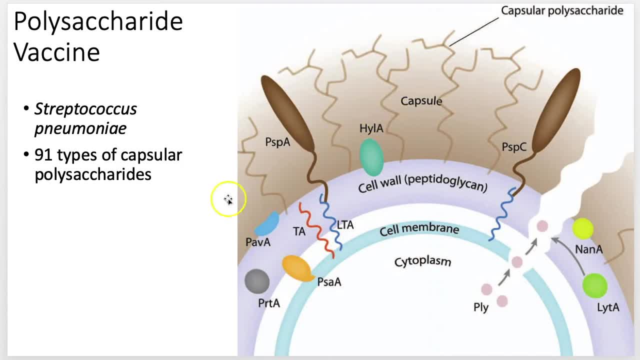 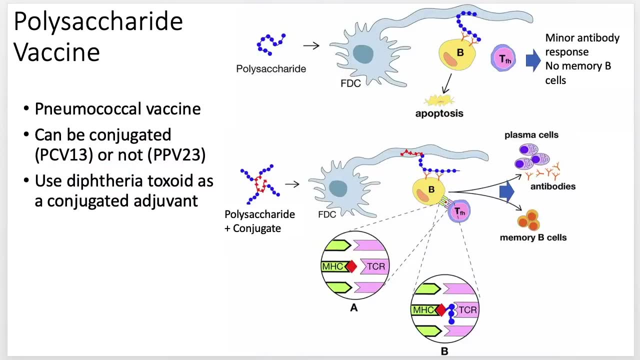 That's crazy. There's so much going on, Okay, And so, uh, it causes a ton of human disease, Like it's really really bad, It kills people, It hurts people a lot, And so, uh, what they try to do was they said, okay, it's the. 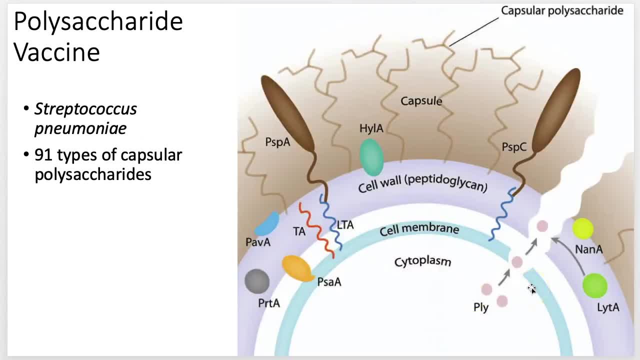 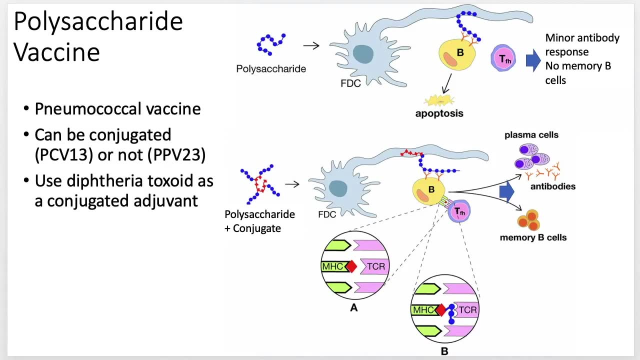 actual proteins on the surface of the bacteria are hiding underneath the capsule. So can we make a vaccine against the capsule? Well, that's a good question. It's it gets a little tricky. So the trick with making uh vaccines that work against uh polysaccharide antigens, um is that. 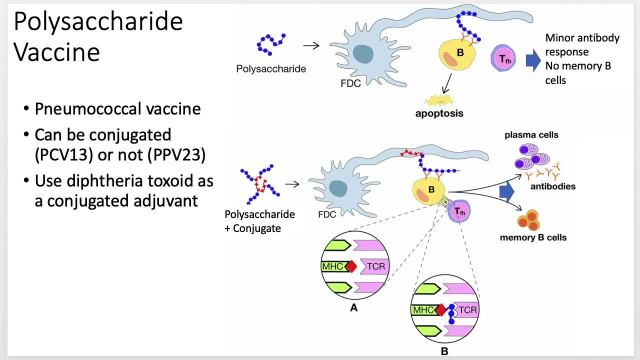 uh, sugar antigens. Okay, So an antigen is any foreign molecule, right, And so you can imagine. we've seen lots of examples of sugars Um the actual like- oh yeah, I have a mannose with a galactose and an N-glucosamine or whatever. Um, the actual structure of sugars um is: 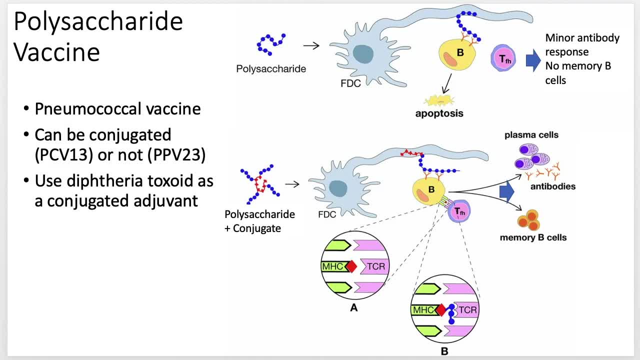 not as uh different between creatures, right, And so it can be kind of tricky to actually uh make, um, an antibody response against a polysaccharide, but you can do it Uh. but the problem is most of the antigens that we deal with as creatures, as humans, as eukaryotes. 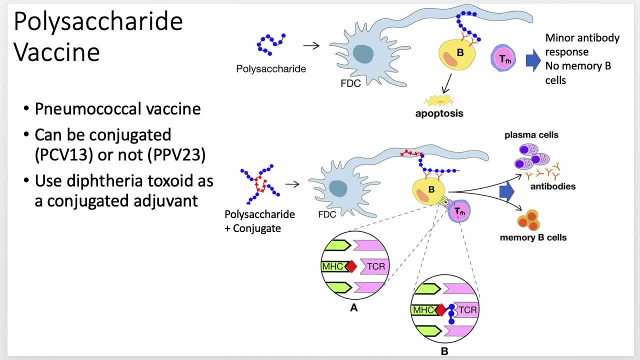 um, that have advanced immune systems like this, um, uh, mammals, I should say, um. most of the antigens that we deal with are proteins, And so, uh, most of the uh recognition machinery. so your MHCs are designed to look for protein antigens, And so, uh, in order you can make. 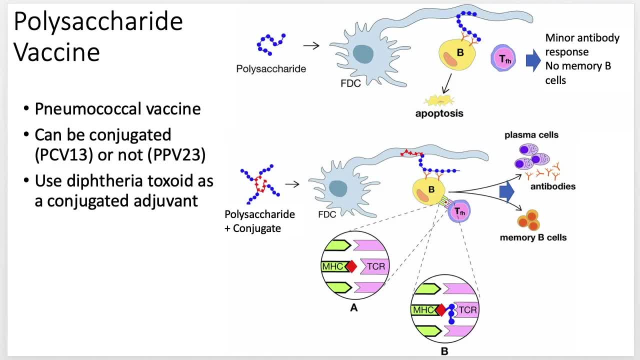 antibodies against sugars, It's just more difficult to actually get the body to do it, And so that's why we conjugate them. So, uh, we take, uh, uh, pneumococcal conjugate vaccine. So that's the PCV13.. This is the one you want to get. Uh, you can get the pneumococcal conjugate vaccine. 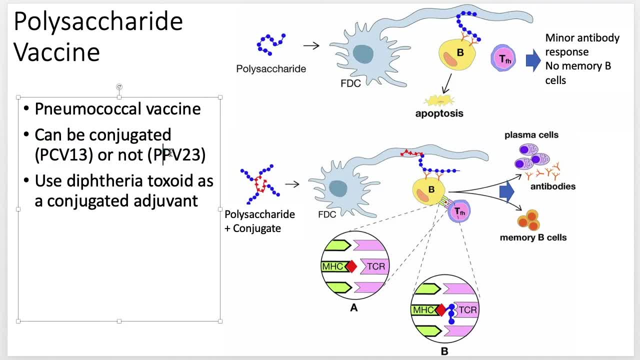 um, it's the non-conjugate, That's just the polysaccharide vaccine. Uh, that's this one. Um, this will only give you passive immunity. So you kind of make some antibodies, but it's not great. 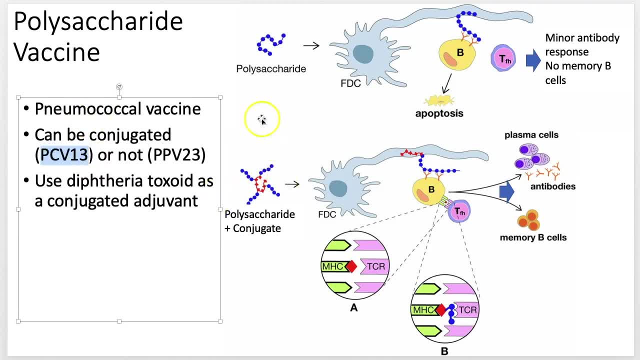 And so what they did was: uh, because the polysaccharides themselves from this capsule are not super immunogenic. they are different enough So we can attack them without attacking the body, but, um, it's really hard to get an immune response. So what they did was they took. 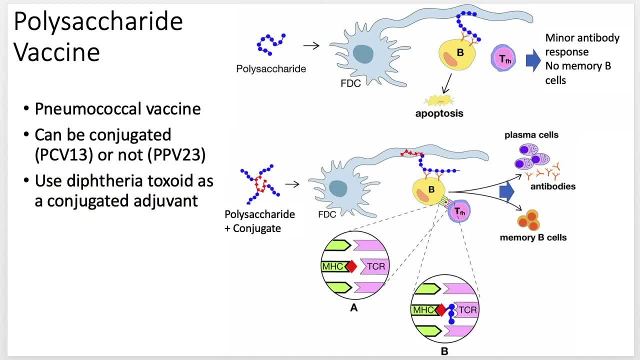 the diphtheria toxin. Okay, And it's a protein, It's the toxin that gets secreted by diphtheria, um and uh, which is a bacteria, and it secretes the toxin and it can hurt you really bad. And so we take a little portion of that, We take the toxin portion off, obviously. 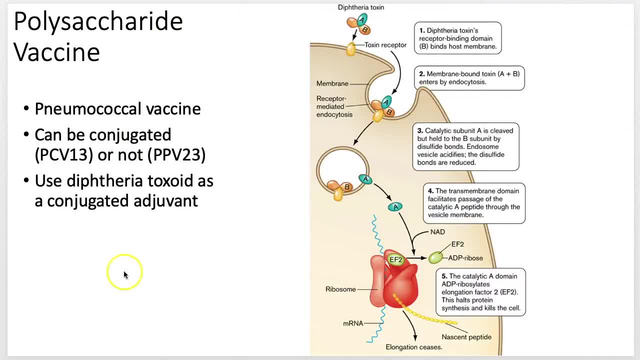 and then attach that to the actual polysaccharide, And so that's kind of what's going on here. So, um, here is the diphtheria toxin. Okay, That's the diphtheria toxin, And so we took off um. 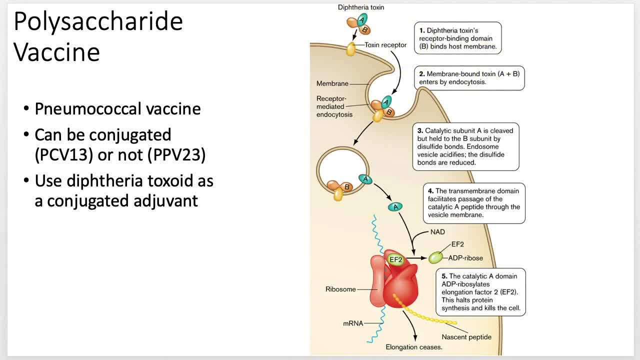 the uh receptor binding domain. Okay, So where is it? Uh, hang on, It's just a sub component of the actual diphtheria toxin, which has two components. The A portion is the one that will actually kill you. Uh, they disable ribosomes, uh, which we haven't really talked about that much. 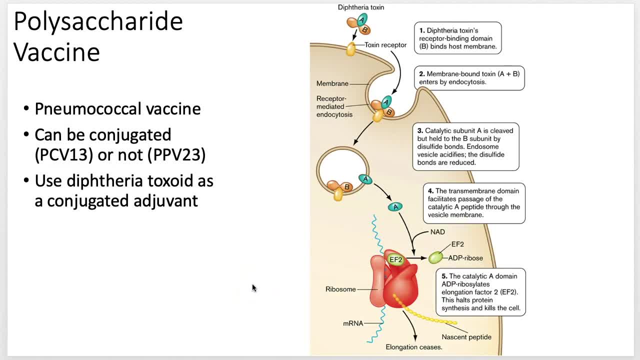 Um but uh, they stop ribosomes from being able to make proteins, So hence why diphtheria toxin can kill you. But we just take a little piece of that. It's super immunogenic. And so when you take just this little protein portion and stick it onto anything, that other thing that you attach it to, 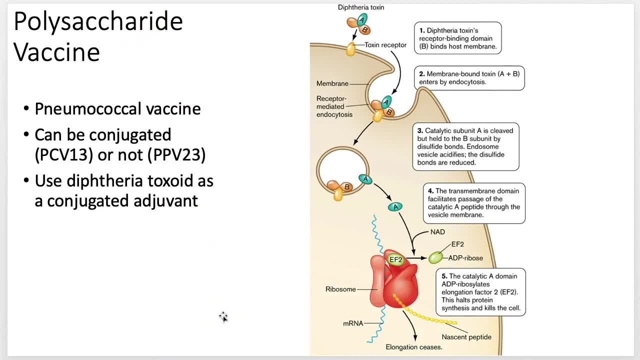 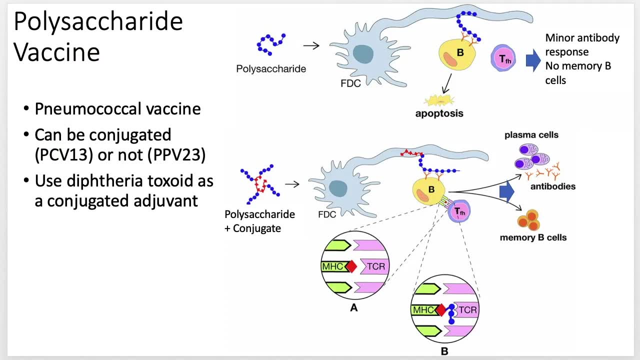 so it could be a polysaccharide or anything else. um can become really immunogenic and you can make antibodies against it, And so that's what, uh, this conjugate vaccine is. So that's what the conjugation actually is. the 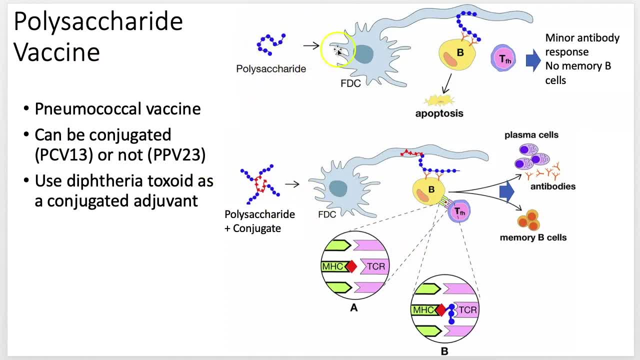 where you're conjugating it, And so that's what this part. So you can have just a polysaccharide vaccine by itself, but it doesn't work super great, Uh, but when you actually do that, you get really good B cell response, which is awesome. Now, the last thing I wanted to show you is a. 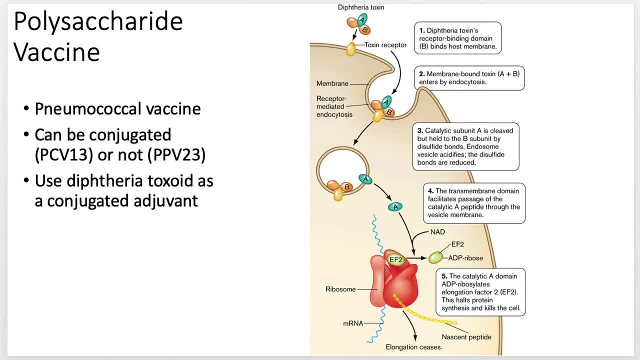 video, and that's just going to end. this video, uh, is a video of HIV. Okay, Cause that was my field for like 10 years. Um, and HIV has a bunch of glycoproteins, And so I wanted to show you a. 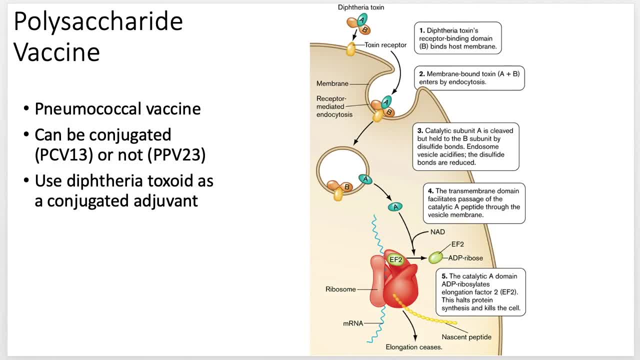 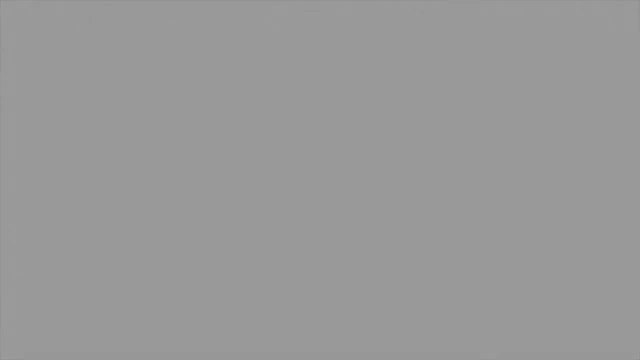 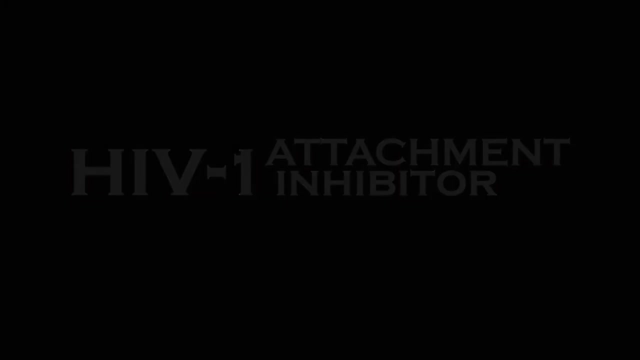 really good, uh well animated video of the glycoproteins and how HIV uses its glycoproteins that it stole from a host cell somewhere else to actually invade another host HIV one attachment inhibitor proposed mechanism of action: Infection of a host cell by HIV leads to formation of new viral particles. death of the infected cell. 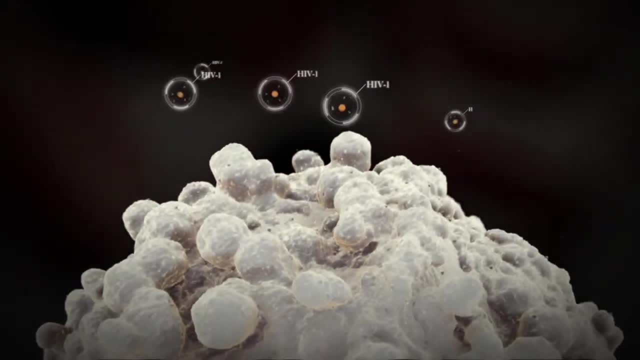 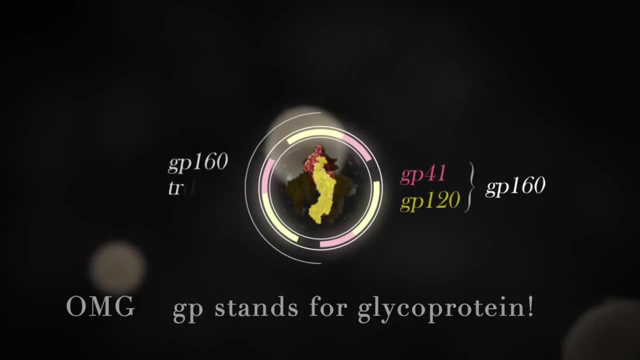 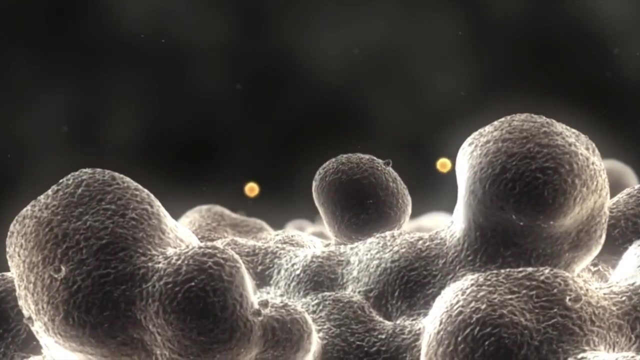 and, ultimately, destruction of the host immune system. HIV particles carry GP one 20 proteins on their outer envelope which play a vital role in allowing the virus to bind to host CD four positive T cells. attachment to the host cell represents the first step in viral entry and infection of the cell. 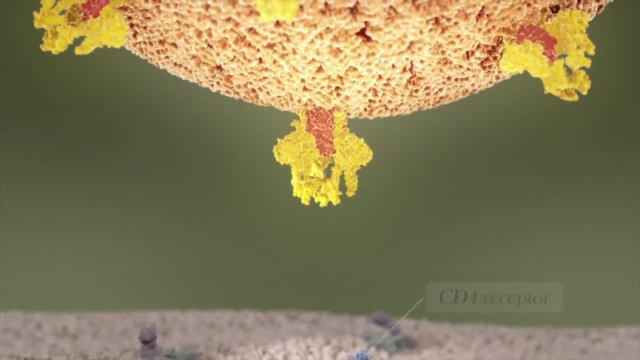 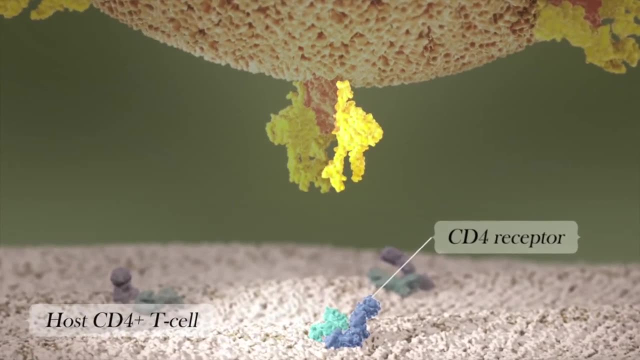 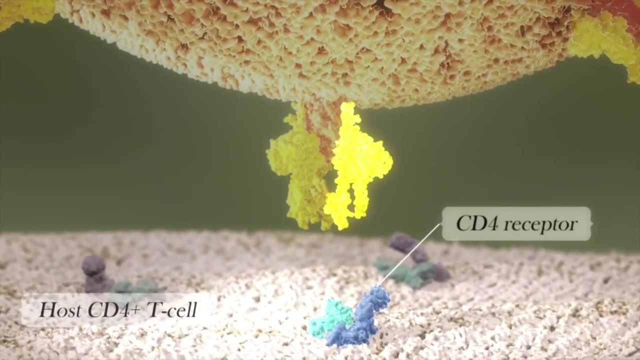 This initial interaction between the virus and the cell, mediated by the viral GP one 20 protein, represents A novel target for anti-retroviral drug development. HIV first binds to the cellular CD four receptor present on the surface of the host cell. CD four binding is mediated by the HIV. 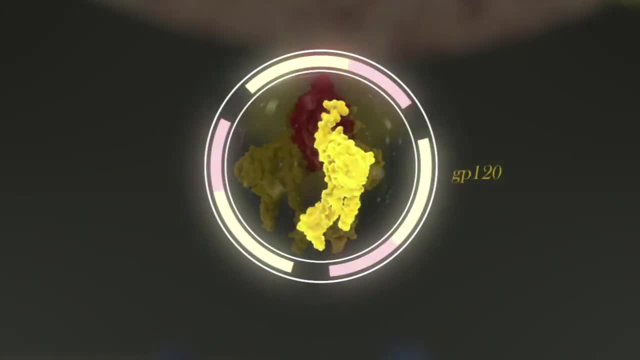 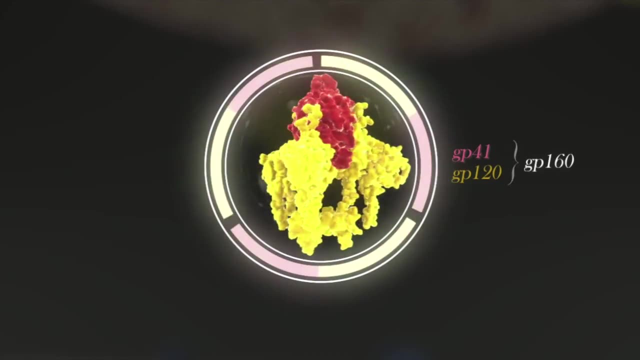 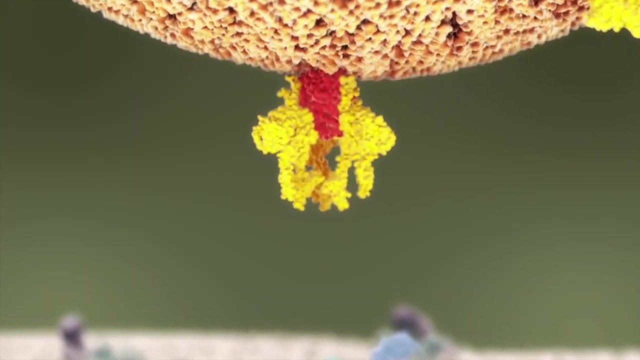 GP one 20, surface glycoprotein, which, together with the transmembrane glycoprotein GP 41 forms GP one 60, which is present as a trimor complex on the viral envelope. in order to enable CD four binding, GP one 20 must undergo a series of internal structural rearrangements. 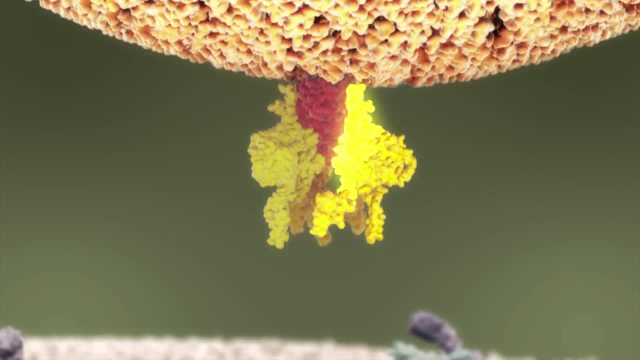 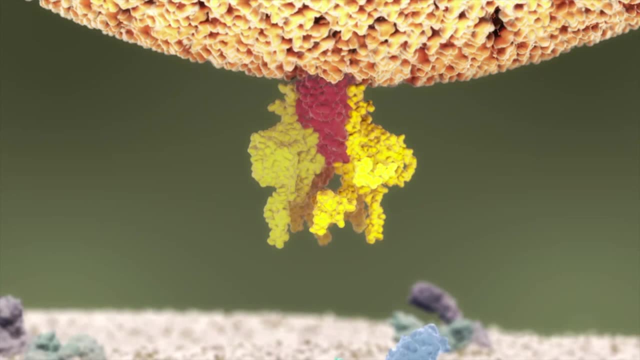 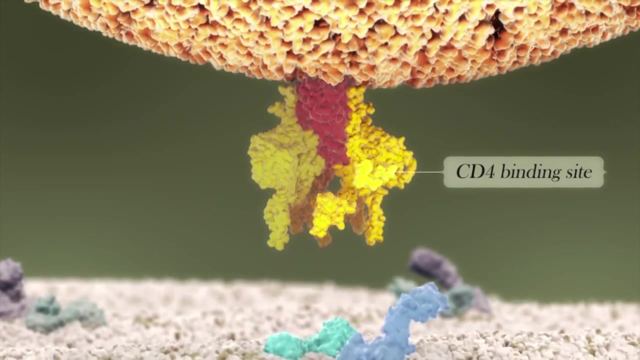 This process begins with rearrangement of the so-called inner and outer domains of HIV, GP one 20.. GP one 20 then undergoes further internal rearrangements in the region surrounding the CD four binding site which enable it to adopt a CD four binding competent state. 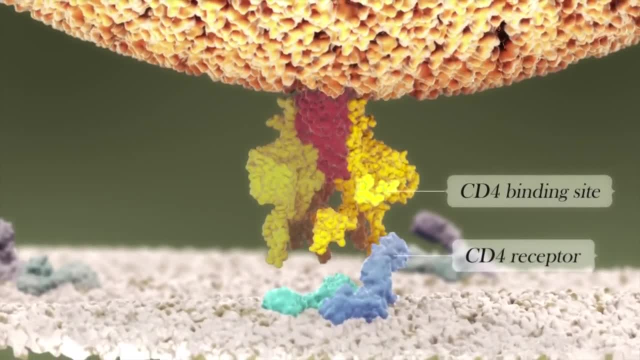 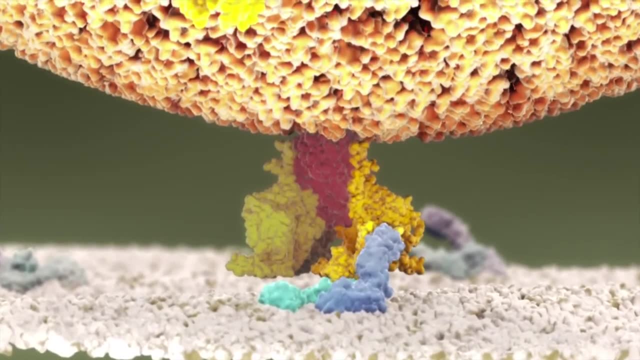 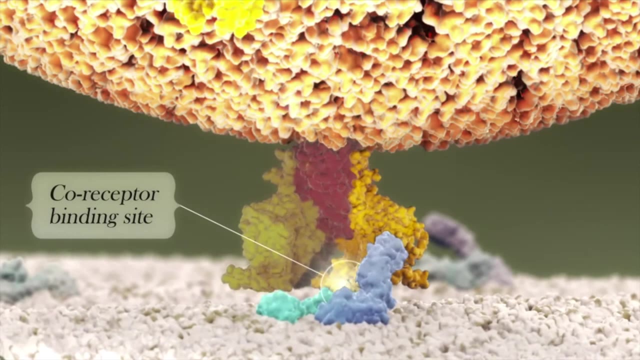 Once in the CD four binding competent state, GP one 20.. Combined to the CD four cell, following binding to CD four, GP one 20 undergoes further folding which leads to exposure of its coreceptor binding site. exposure of the GP one 20 coreceptor binding.